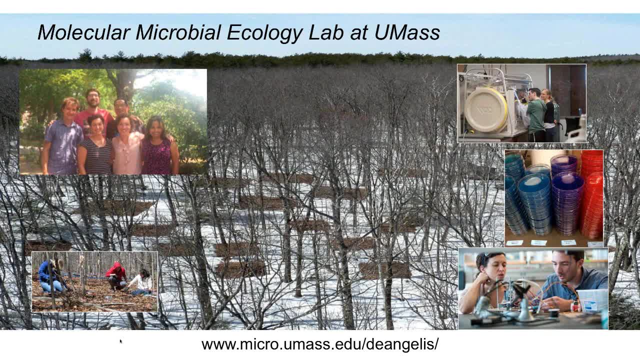 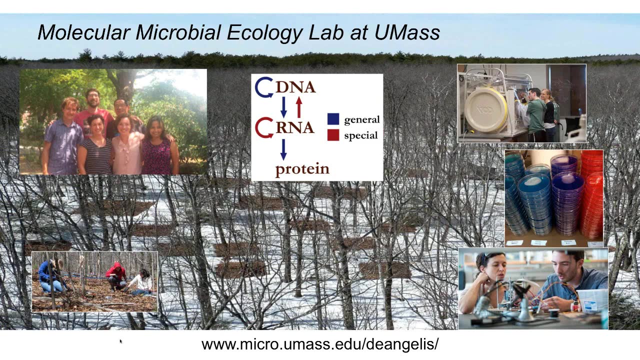 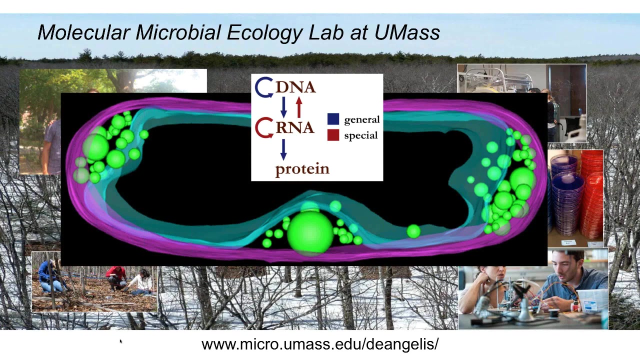 So I'm going to just spend a couple of minutes introducing myself. I am a professor at UMass, Amherst, and I run a lab. I call it a molecular microbial ecology lab. So molecular means that we study molecules in microbes. So maybe you're familiar with the central dogma of biology, which means all organisms have DNA. The DNA is transcribed to make RNA, The RNA is translated to make protein and the protein does all the business of cells. And by sequencing these different elements of DNA and RNA and protein, we can know about microbes, which by definition are any organisms that we can't see, and know what they're doing, and we can know their 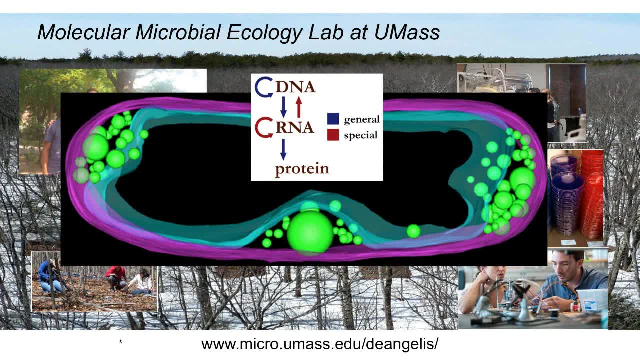 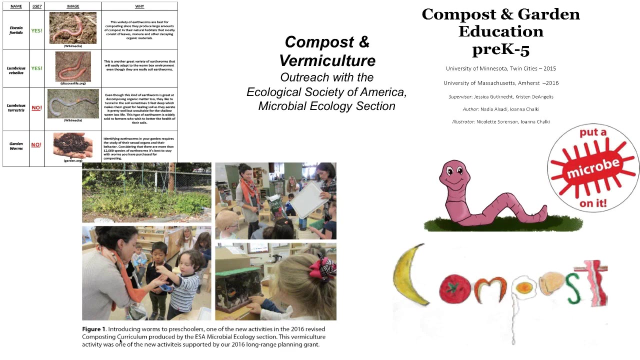 ecology, their ecology being how they interact with other living organisms, like other microbes and plants, and how they interact and respond to and shape their environment, including environmental stresses that might be associated with climate change, And so that's really what we do in the lab. 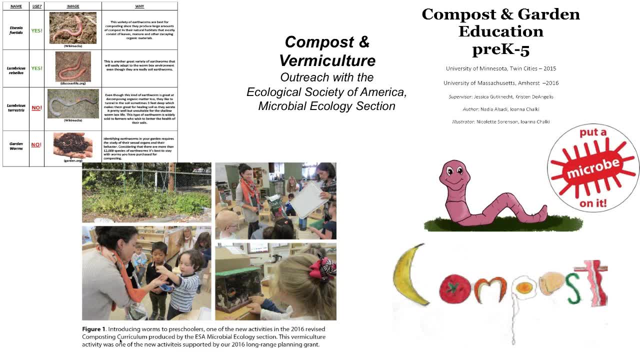 As part of our lab work. we also do a lot of outreach and I'm just showing you an example of an outreach project we did last year: manual. that was intended for just regular citizens to incorporate more microbiology into their plant waste that they might generate in their homes or in 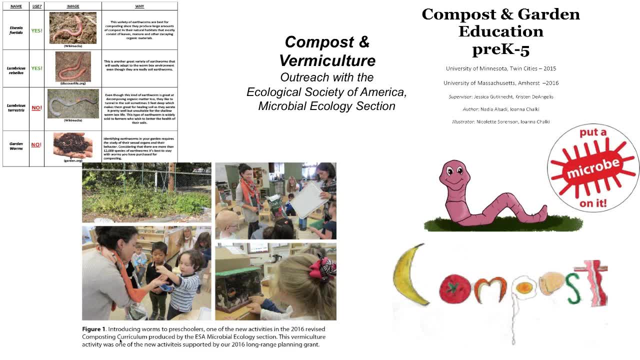 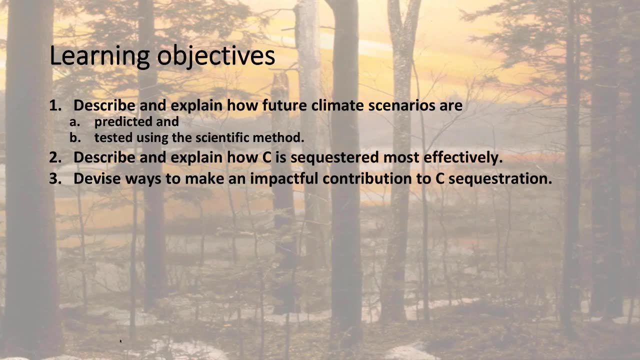 their yards, and part of this was, you know, creating like a key so that you can understand more about the worms, and then we also donated some vermiculture kits to local preschool. so so that's that's me, and that's what we do, and so now I'm gonna show you and talk about the, the learning objectives. this is what 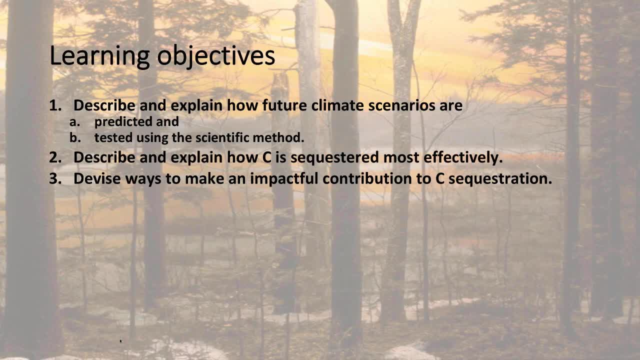 I want to accomplish with this webinar and at the end of this 50 minutes, hopefully you will be able to describe and explain how future climate scenarios are predicted and tested using the scientific method, and when I talk through this part, I'm going to give you an example of how we use the scientific 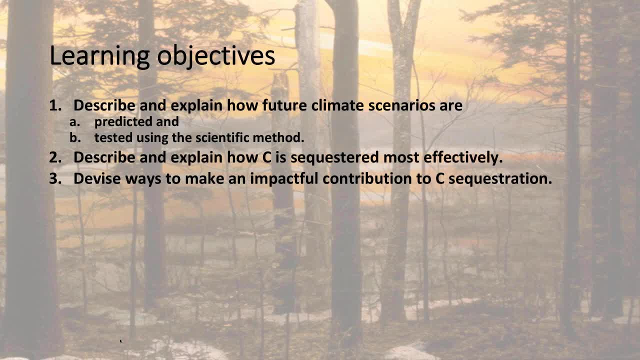 method to understand the microbiology of climate change. two: by the end of the seminar, you should be able to describe and explain so conceptually how carbon is sequestered most effectively in soils, and I'm going to talk about some different studies that tested different scenarios to see. 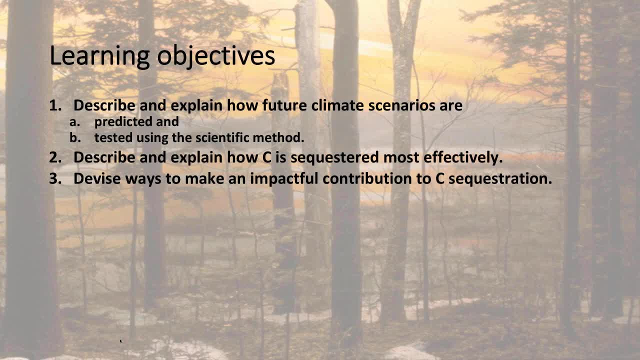 how that could change the effectiveness of carbon sequestration. and then three, I'm going to talk about some ways that that you personally could make an impactful contribution to carbon sequestration, based on new public applications coming out of the scientific community. so so, to begin with, 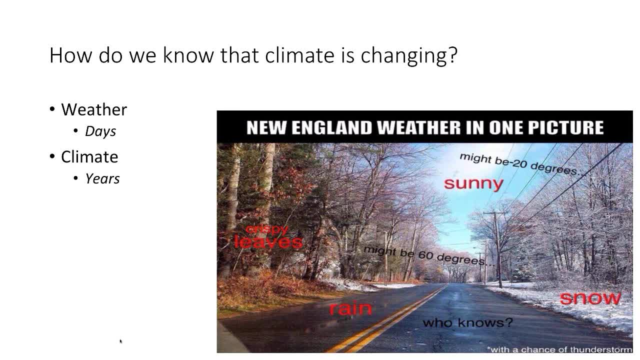 how our future climate change scenario is predicted. so just to make sure that we're on the same page here. climate and weather are related and really the difference is in the time scale. so the climate is how the what the weather is like over long periods of time, and so the weather sort of happens over days. 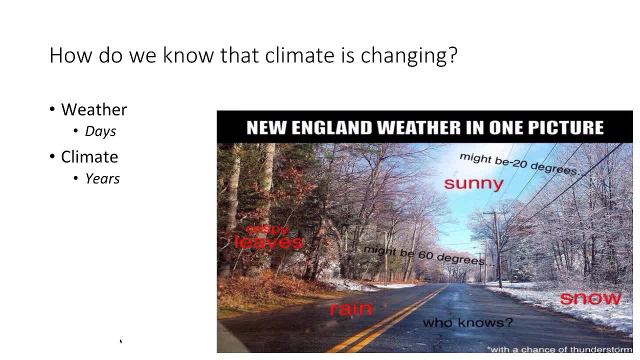 and maybe you know that we're actually really good at predicting the weather right now, and so you read a weather forecast, even in a place like New England where the weather really changes a lot. you know, in the morning, between the morning and afternoon, we're getting better at predicting the climate. so what's the 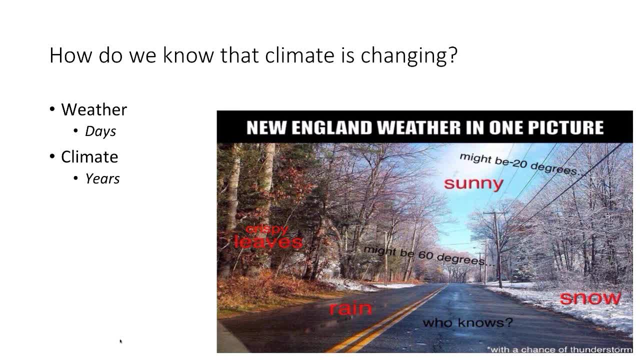 weather going to be like next year, in five years, and so so, even though they are separate, they are related, and one sort of interesting thing about today and, you know, 2018, is that we're starting to see some climate change impacts that are affecting our own weather in terms of, you know, breaking temperature records. 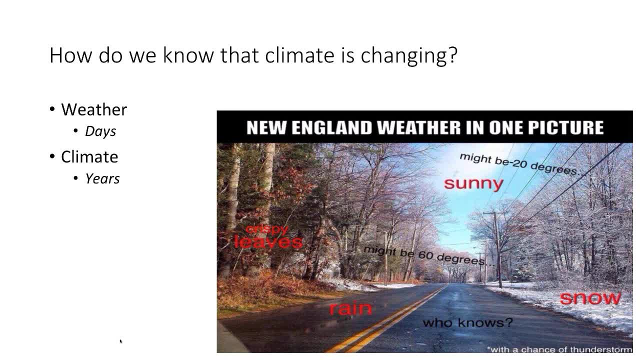 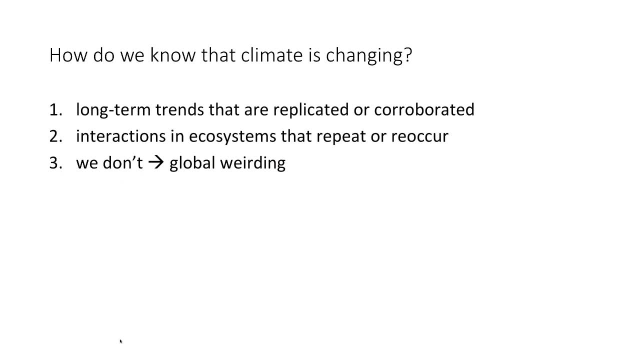 for example, or having record like wet winters, wet summers. so how do we know that the climate is changing? there are really three ways. one: there are long term trends that we can predict that are replicated or corroborated in different ways to their interactions, and ecosystems that can repeat or reoccur. so 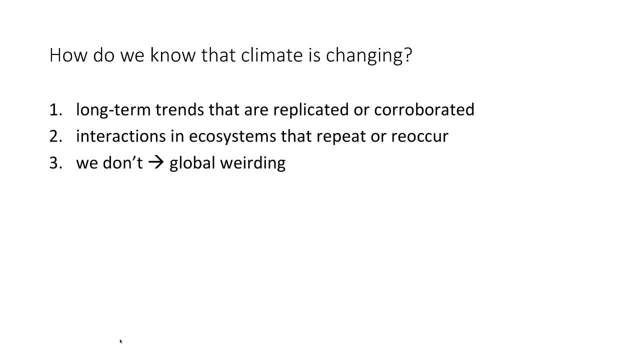 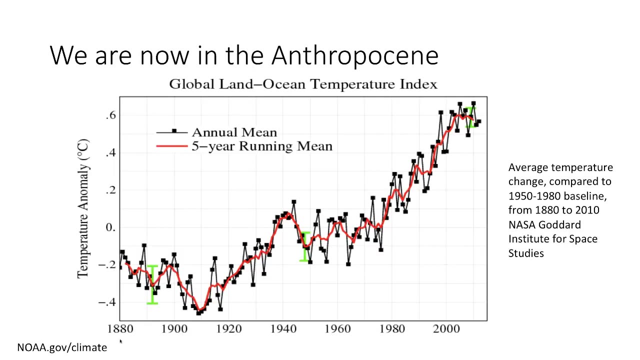 you know, we think that we see something and then it happens again, and then three part of it is we don't. there's an element of unpredictability, and sometimes you go call that global weirding, this idea that there's always going to be some element of the system that we don't quite understand yet. so a lot of 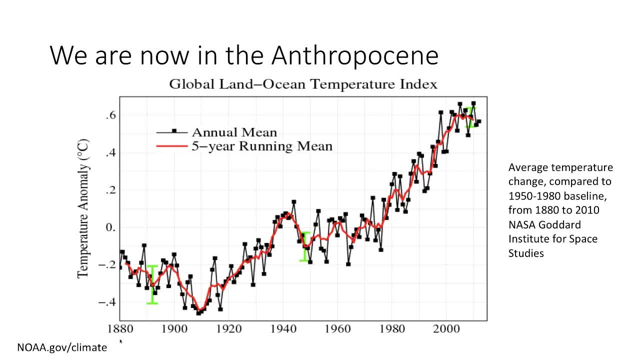 scientists now think that we're in the Anthropocene. the Anthropocene it's this proposed new epoch that describes the time of the Earth's history in which is characterized by people having an impact on the climate and the geology and the systems of the earth, and so this is a 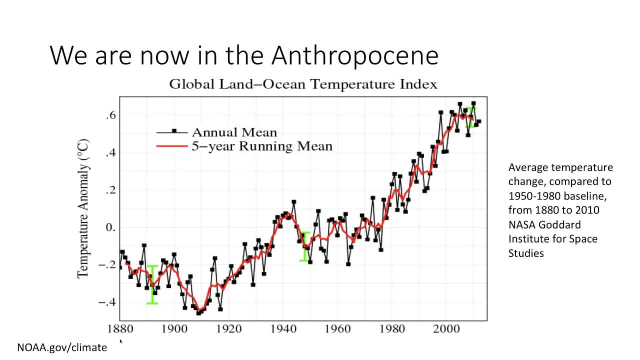 really interesting idea and still a little bit controversial: this idea that humans are have such an impact on the earth that we're essentially a geophysical force. but the data it really proved that this is true. so what I'm showing you here, this is from the NOAA website and this is the temperature anomaly where the average 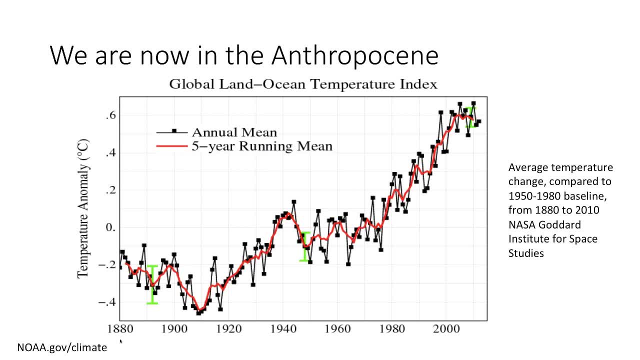 temperature change is plotted on the y-axis between 1880 to 2010, and this is the average change compared to this baseline that is established, just sort of defined, as being this time between 1930 and- sorry, 1950 and 1980. so take the. 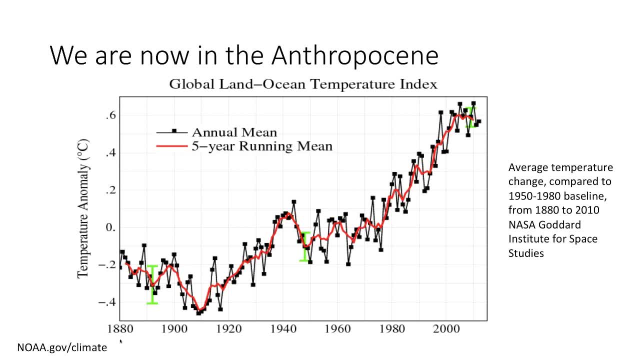 average of the temperatures between 1930, 1950 and 1980 and then compare what the average temperature actually was in those different years and you can see that, compared to that, 1950 to 1980 the temperature anomaly was below zero and now it's above zero and heading up. 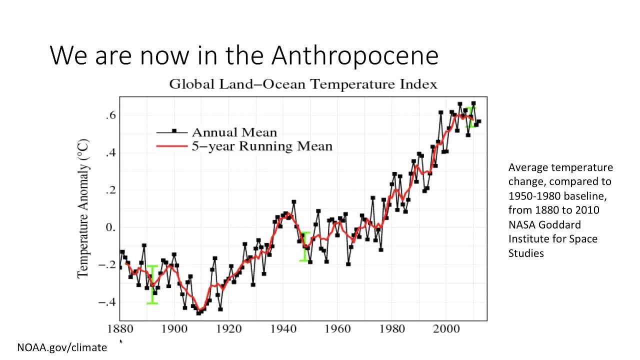 towards one degree temperature increase compared to this mid-1900s level, and so this is a trend that we're seeing repeat, we're seeing continuing and actually accelerating. just last week the IPCC came out with a new report, this 1.5 degree report. that says that we're pretty much committed to. 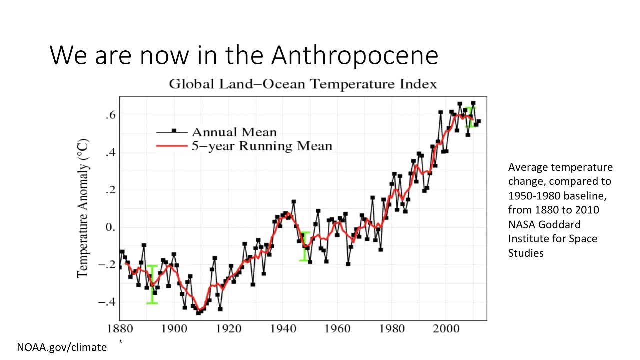 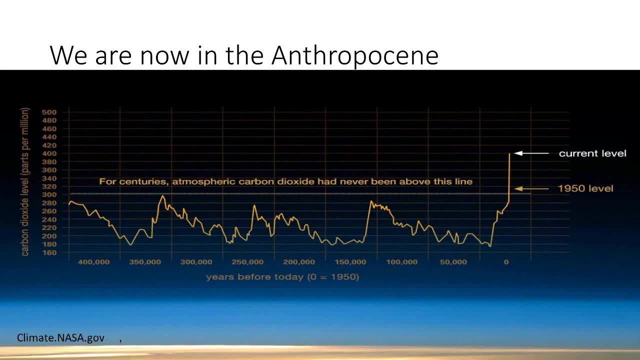 at least a one degree increase in temperature. so this is a real, a real trend that is not slowing down, and part of this is coming from carbon dioxide, and so carbon dioxide does fluctuate, naturally, but our focus here is on the amount of carbon dioxide that we have and we're doing. 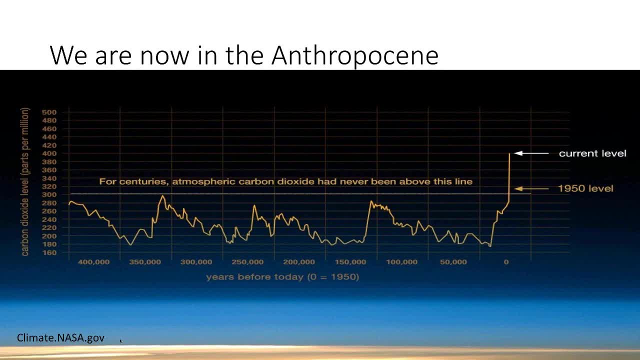 this to help your stop warming and other things, and so the good news about the carbon dioxide report was that every year in the last year, the carbon dioxide levels have risen even higher, and every year, for example, compared to the annual climate change results, the climate change results have increased, and for 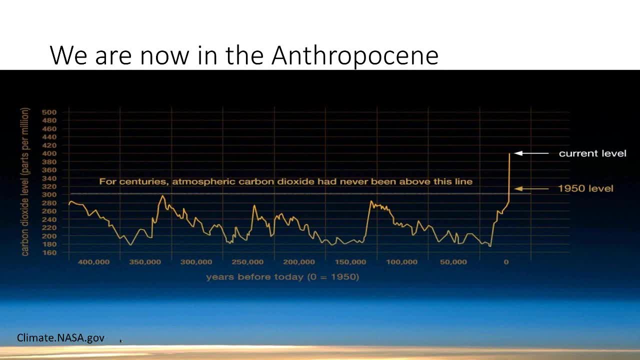 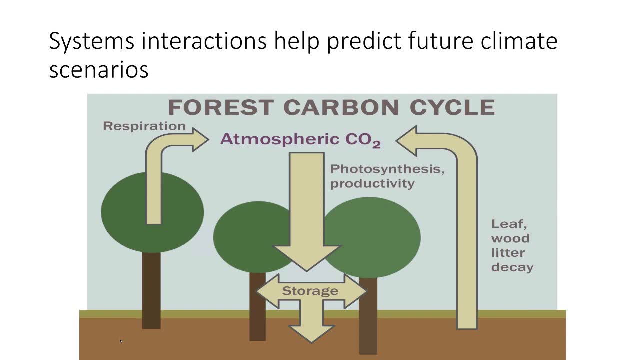 example, we have a high level of carbon dioxide here now in the United States sink right now for this carbon dioxide that's coming from these anthropogenic emissions, And so you know, in a natural system that maybe you're all used to thinking about, where you have trees and grasses, the amount of carbon dioxide. 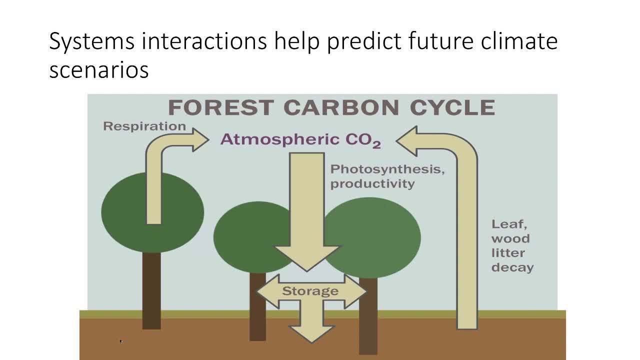 coming out of the system is pretty much in balance with the carbon dioxide that's being sequestered by the system. So in a natural system where there aren't, you know, cars and factories, there's respiration that comes from plants and then there's respiration that comes from leave, wood, litter, decay, that. 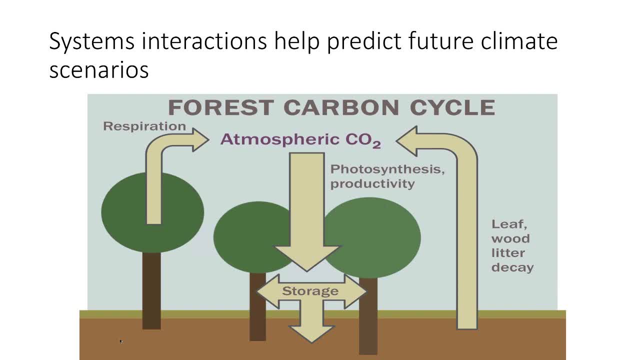 comes from the soil microbes. That's my interest. The amount of carbon dioxide coming from plants and soils is about the same as the amount of CO2 that's coming back into the system, being fixed through photo synthesis, And that CO2 carbon is, once it's fixed, it's stored in trees and it's stored. 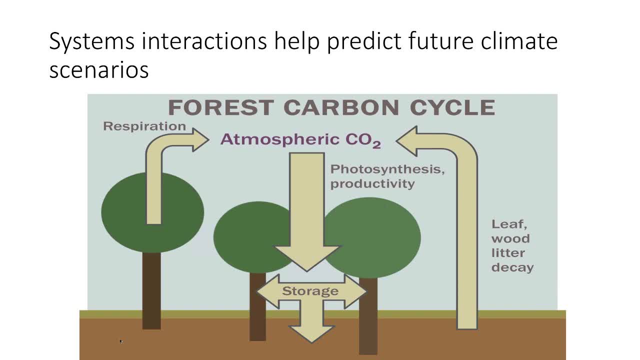 in systems Shown inント Drive Times soils. So this is a very simple example of the carbon cycle And by mapping out the fluxes, or how much carbon is moving from one state to another, and the pools of carbon, how much carbon is in the CO2, how much carbon is in the plant biomass. 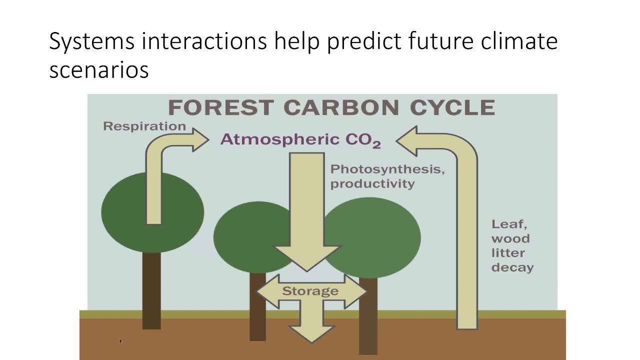 this forms this very simple carbon cycle, this biogeochemical cycle, And by measuring these pools of fluxes we can understand how systems work and how stresses affect ability to store carbon or release carbon into the atmosphere. So this is a simple model, And where we're going is. I want to give you a 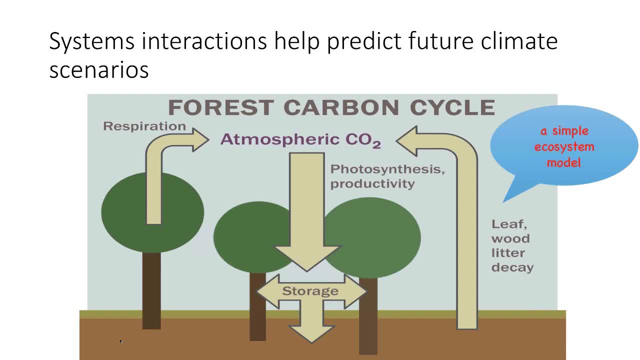 sense of how the small microbiology stuff that we work on can scale and inform these climate models on this global scale. So here are the pools, here are the fluxes. so the pools are places where carbon is stored, the fluxes are the arrows, this measurement of movement. 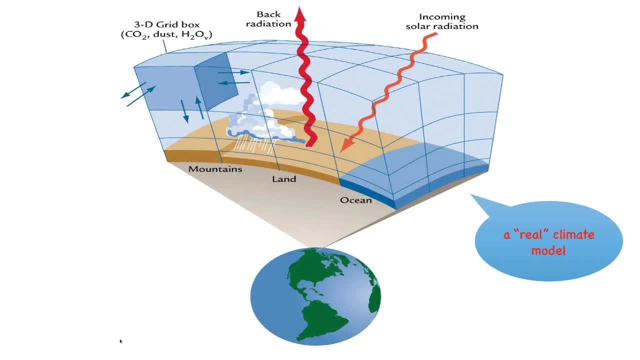 And so a real climate model might look something like the simple climate model, but the pools and fluxes might include things like carbon dioxide in the air, land and oceans, And so the individual climate models are set up where they have these little boxes where you can measure fluxes coming in and out. 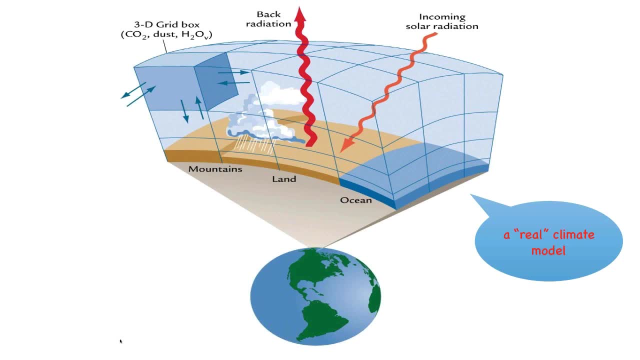 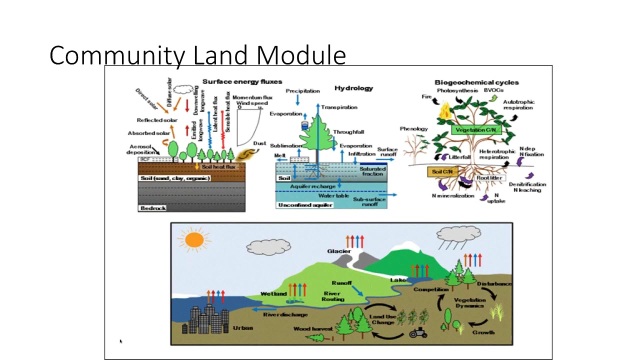 and then look at the carbon cycling in the box and the exchange between the boxes and in that way you can scale the system from a little ecosystem, you know, a little foresight, up to a global level. And so the resolution of this is poor, so I apologize for that, But this is an 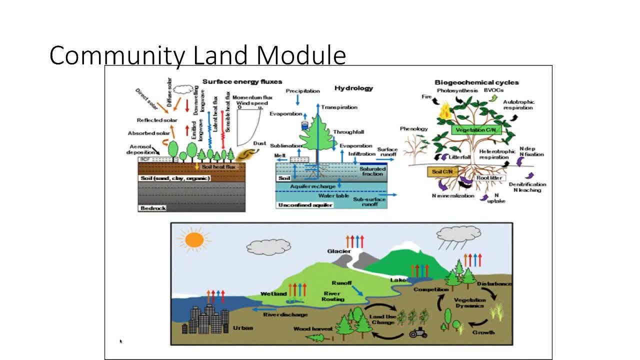 actual diagram of a global climate model called the Community Land Module. And the Community Land Module measures pools and fluxes in terrestrial systems, in aquatic systems, between soils and plants, and then uses this sort of grid box system to allow the different ecosystems to interact with each other And in that 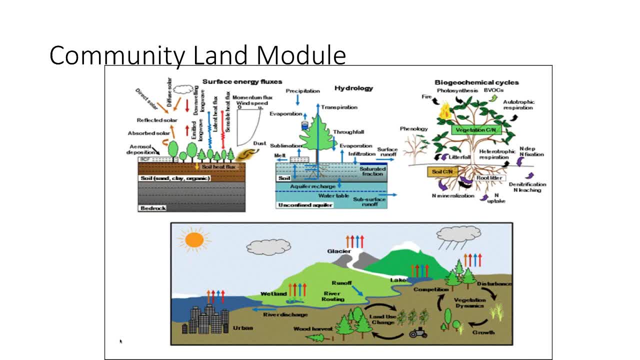 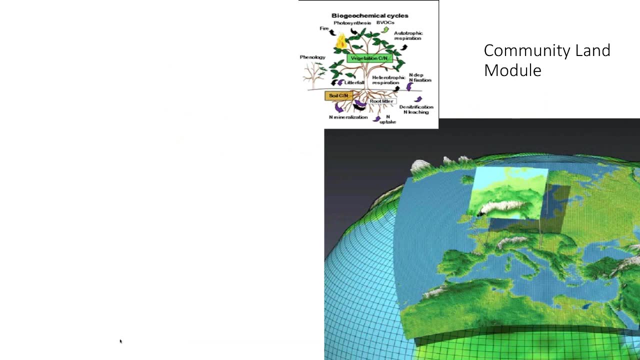 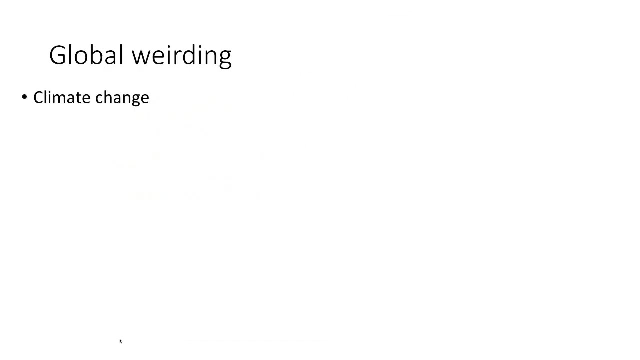 way you can scale up from knowing sort of specific interactions about how plants or forest systems might respond to land use change, by deforestation for example, and how you could scale that up to a global system. So you have sort of an individual component of the Community Land Module and then that sort of fits. 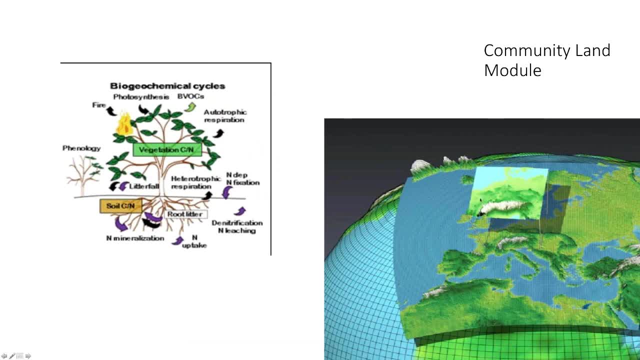 in to this grid. So hopefully you can see sort of on the side here where you could imagine looking at pools and fluxes and plants for just a single grid and then interacting grids scaling all the way up, And so this is one way that we 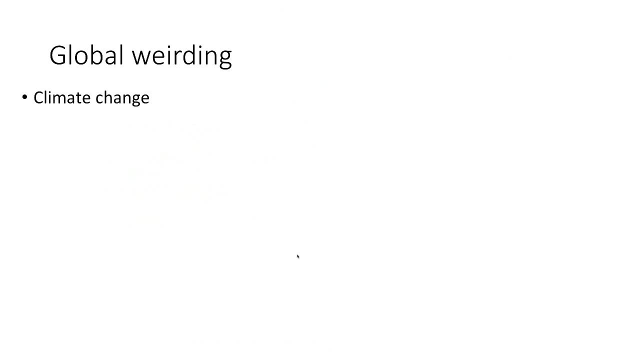 know that the climate is changing is by mapping out the carbon cycle, making predictions about what's going to change and then sort of scaling that up and then testing ourselves by doing things like measuring carbon dioxide and atmosphere. But there's always this element of global weirding this. 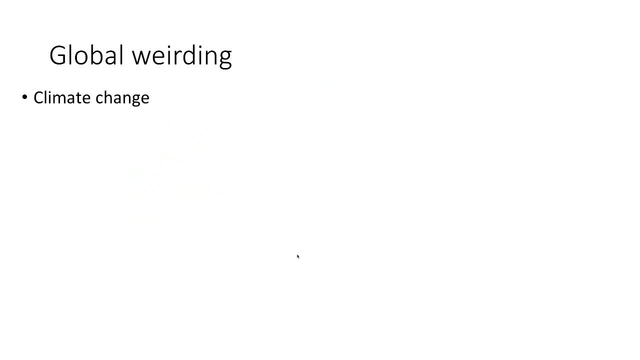 unpredictable element, and especially as we sort of continue in time to have our human emissions, anthropogenic emissions, unchecked. We're really heading into a time where a lot of scientists feel- and I am one of them- that climate change isn't really the right way to describe what's happening right now. We're really 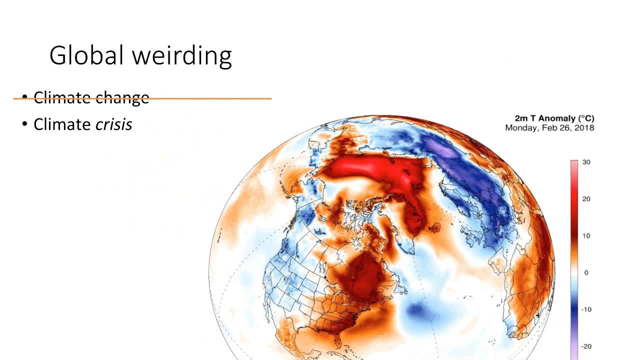 in a climate crisis. This is from last February, when I met the ELA organization folks in person, and what was happening now is that the Arctic was experiencing a two degree increased temperature anomaly than normal, And so we're entering into this time in our planet where we just don't know what's going to happen when, for. 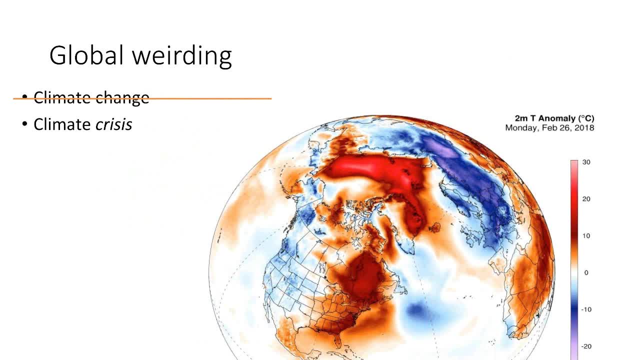 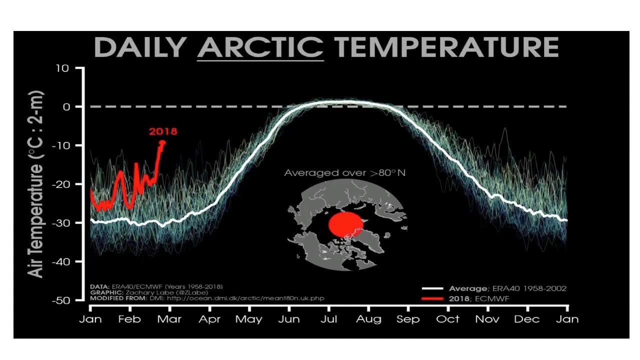 example, we lose all of our Arctic sea ice. even in the winter, It's almost certainly going to increase sea level, for example, and that's what models predict, But we've never actually lived through this before. We have one planet and we just don't know. This is. 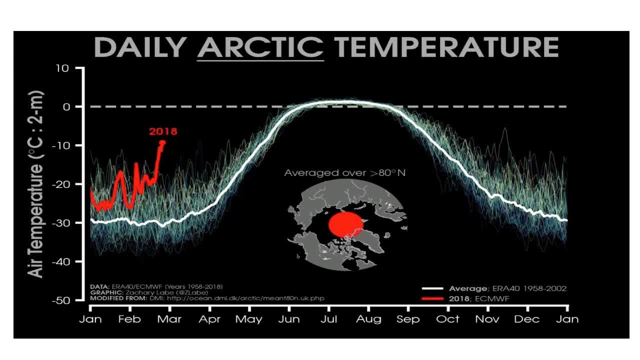 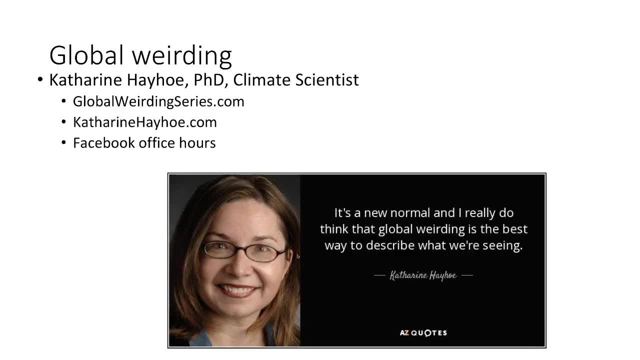 another measure from last winter of this daily Arctic temperature. that's really rather alarming, And so this concept of global weirding is being explored by a climate scientist named Katherine Hayhoe, and I just love her. She has this web series called globalweirdingseriescom. 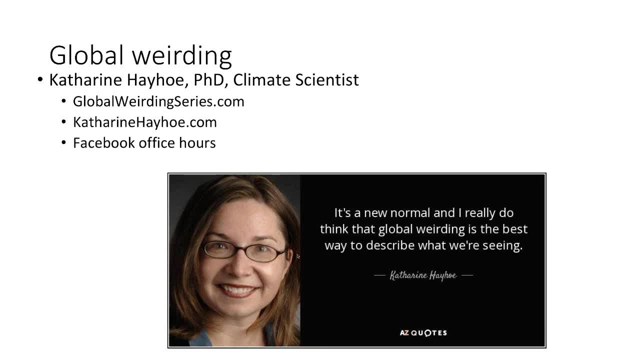 She has office hours on Facebook, so if you want to learn about this, you can find her on Facebook and tune in, And she does these live office hours where she'll take questions and talk to folks- just any kind of question She's. 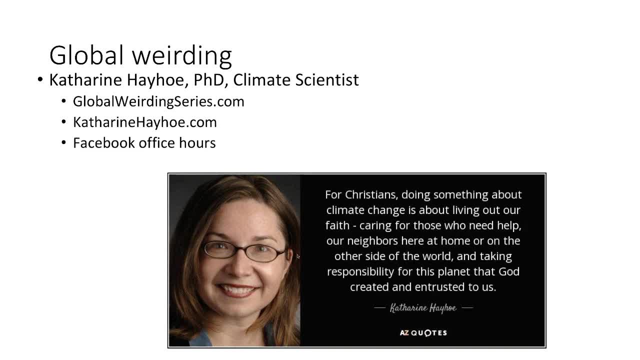 really interested in helping people understand what's happening right now, And so you know what she says is it's a new normal, and I really do think that global weirding is the best way to describe what we're seeing, And for those, 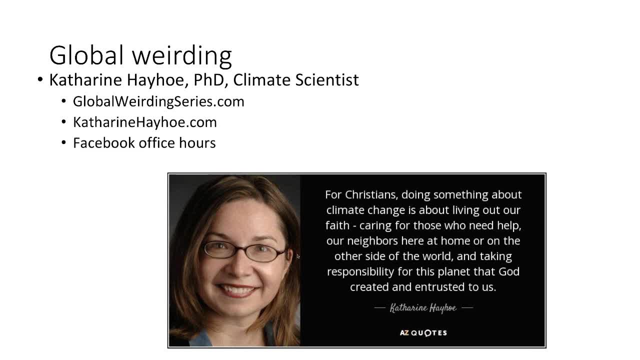 of you who are religious. she's also Christian and she's really interested in this idea that it is part of her Christian faith that it is important to take care of those who need help, and that includes on our planet. So if you're interested, she's. 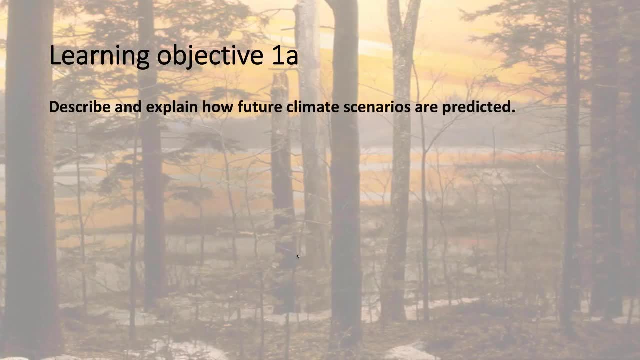 definitely someone who is worth checking out for this specific idea. So I just talked to you about how future climate scenarios are predicted. These long-term trends are predicted and then replicated. We can look at interactions between ecosystems and see how they repeat or reoccur. 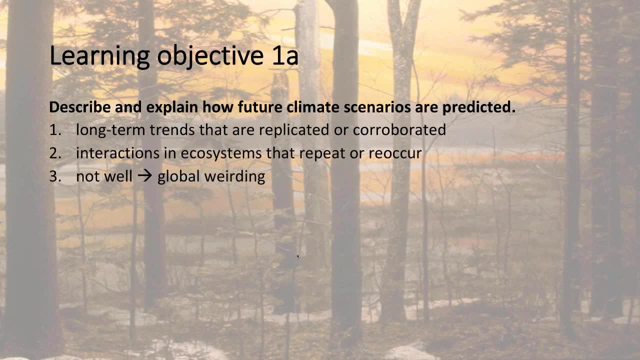 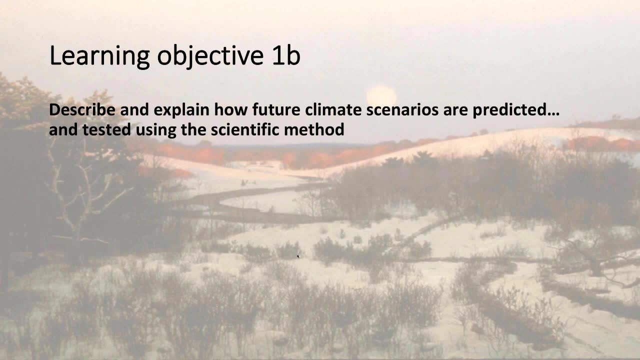 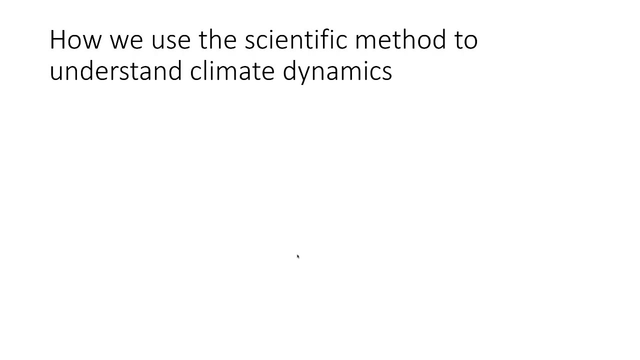 through different ecosystems, And then there's always this element that we don't quite understand, which is global weirding. And so now I'm going to move on to this next idea, where we're going to talk about how to test future climate scenarios using the scientific method, And so the scientific method is. 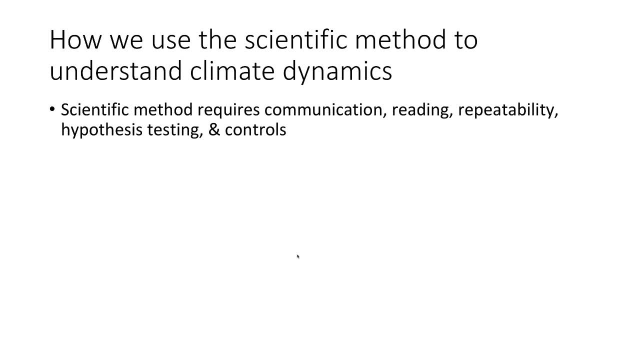 something that really anyone can use. All babies use this to learn about their world. It requires communication. For an adult, it requires reading. You want to repeat your results And basically you come up with an idea, a hypothesis. I think things should work this way, And then you test it, And then you 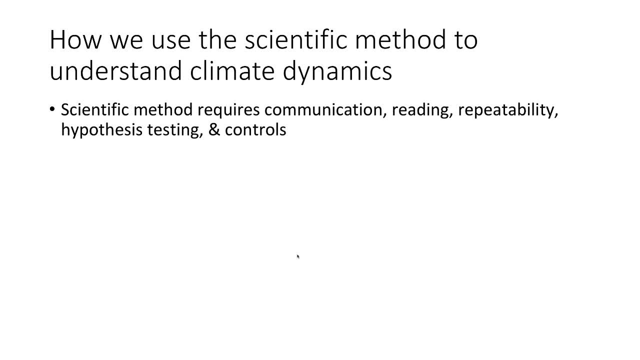 reevaluate. Was I right about that? And then you always want to include some kind of controls. Well, maybe you know there's a reason why this would happen, and so you want to control for that. And so research on climate and soils happens on many scales. The micro scale is where I'm. 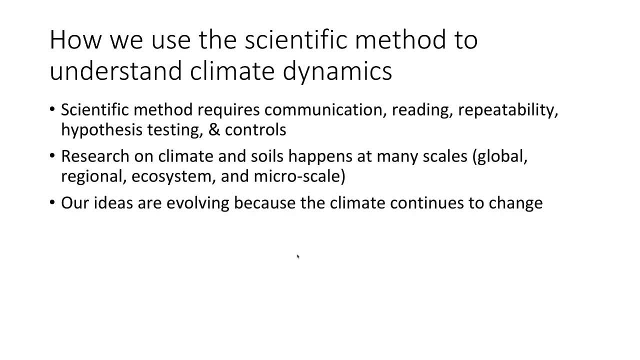 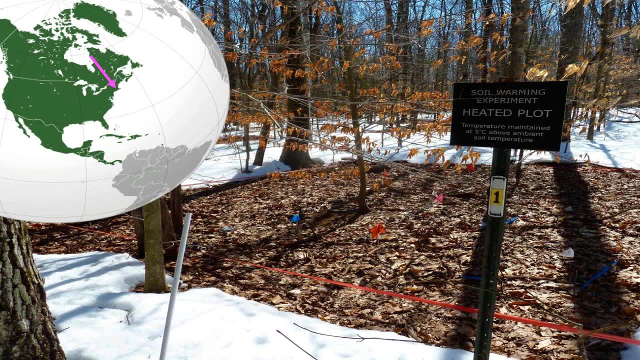 talking about what we've been talking about these global and regional scales so far, And our ideas continue to evolve because the climate continues to change. So now I'm going to talk about the research in in my lab. Since I started at UMass in 2011,, I've been working in this long-term warming experiment And it's a 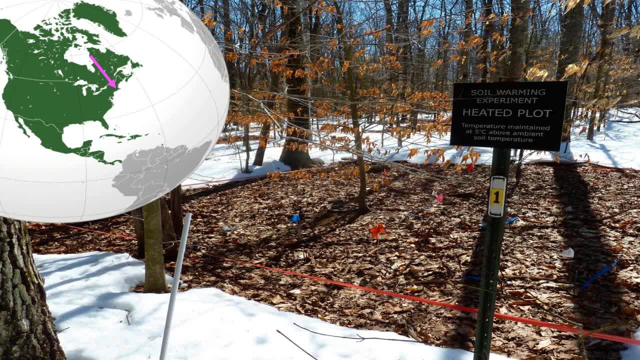 climate change simulation. that was a study that was done in the United States And it was a study that was done in the United States, And it was a study that was done in the United States And it was a established in 1991.. So that's 27 years ago, And what my colleague did was they. 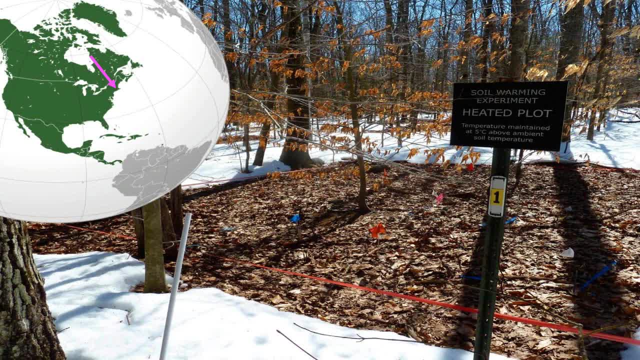 set up these field sites, And you can hopefully see the plot here that is delimited by these orange, this orange tape And what they've done actually, and so I just want to point out this is in Petersand, Massachusetts, at the Harvard. 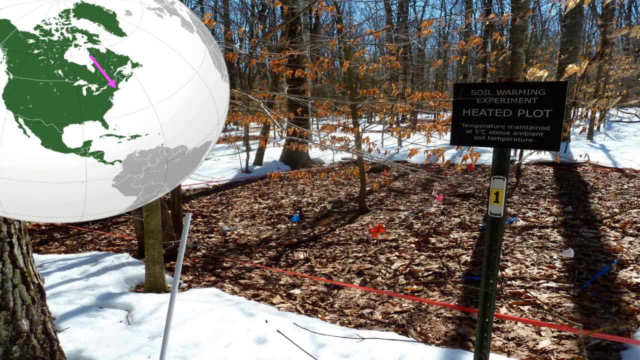 Forest, which is central Mass, And what they did was they buried resistance cables into the ground at 10 centimeters depth. And these resistance cables, they're heating cables. Maybe you've seen a football game like a Green Bay Packers game, where it's the football game is happening in the winter. 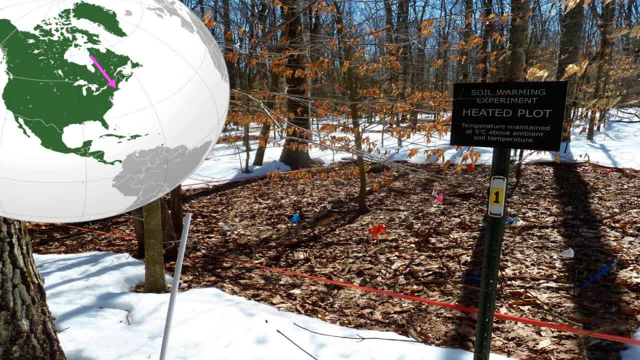 outside and there's lots of snow coming down and snows accumulating on the sidelines and on people's hats and coats, but somehow the field stays green And it's because of the same technology, these varied heating cables. So there are thermistors attached to the cables that are spread out, you know, every 10. 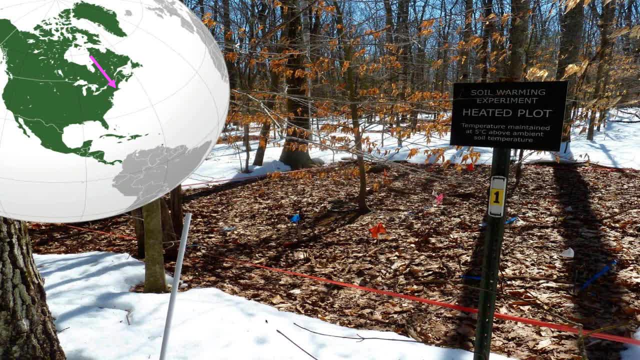 centimeters throughout this plot and they're connected to a data logger and thermistors in control plots And the data feeds back every 10 minutes to adjust the amount of electricity coming to the cable so that these heating plots are maintained at 5 degrees above ambient soil temperature all year round. 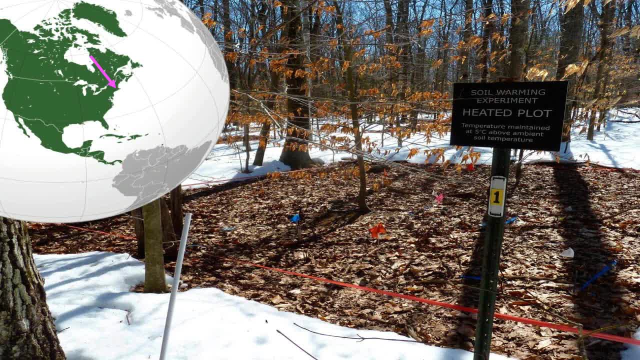 Now we don't usually study the soil dynamics in the winter and that's probably because the ground is frozen. there's not a lot of biological activity, so it's just a challenge. But I like to show this picture of winter because it really shows you how much a 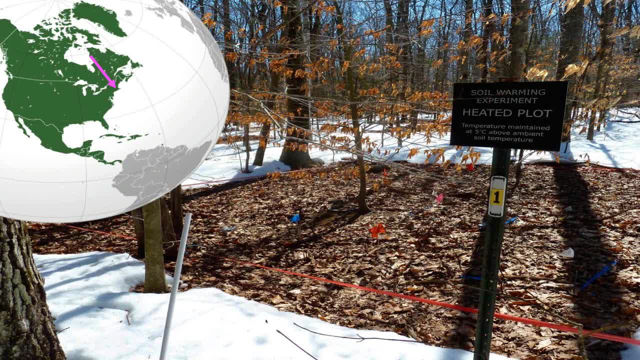 future climate change scenario like 5 degrees might really affect an ecosystem. Now, 5 degree global temperature seems pretty unlikely, right? We just talked about that. we're pretty much locked into a 1 degree temperature increase and that's a global temperature increase And we're looking at 1.5 degrees. 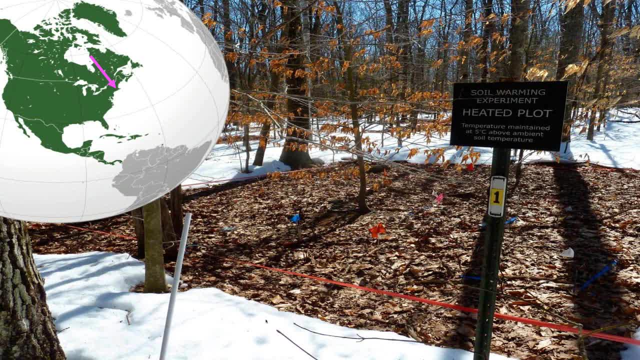 unless we really make some drastic changes in the next decade. So 5 degrees is a lot, but remember I showed you that picture of the Arctic temperature anomaly. that was 2 degrees. So climate change is affecting different ecosystems in different ways, at different rates all over the world, And one of the things 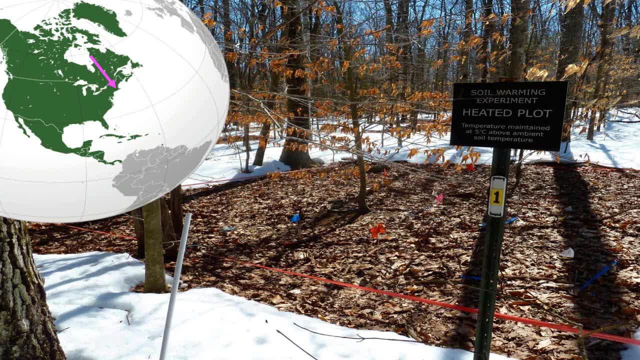 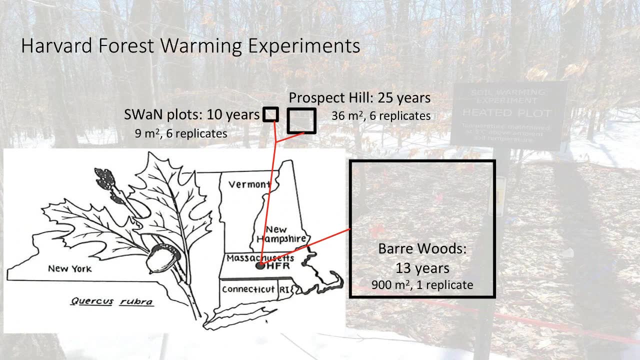 that we are trying to do as a scientific community is understand how climate change is affecting different ecosystems differently and really focus on the most sensitive ecosystems. So there are actually three warming experiments happening at the Harvard Forest. This longest-running experiment that I'm going to talk to you about today is now. 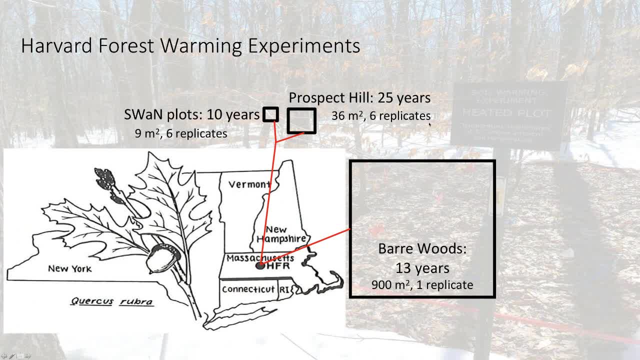 28 years of warming. There are six replicate plots, six heated plots and six control plots that are 36 meters squared. There's another experiment that's been running only for 10 years nearby. that's actually a soil warming by nitrogen amendment experiment. And then there's a third experiment that's been 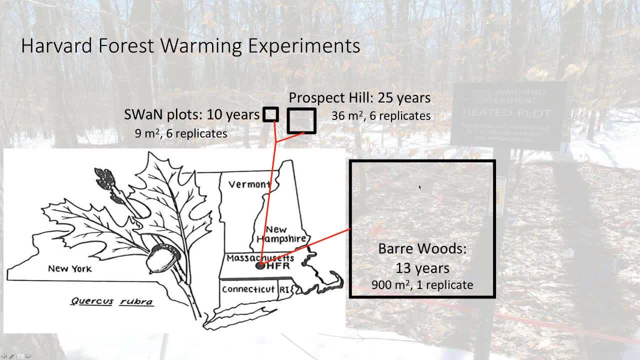 running for 13 years. that is a one large mega plot, And it's only in this Barry Woods experiment that we can really look at this interaction between plants and soil, which is really important. But so today I'm just going to talk to you about 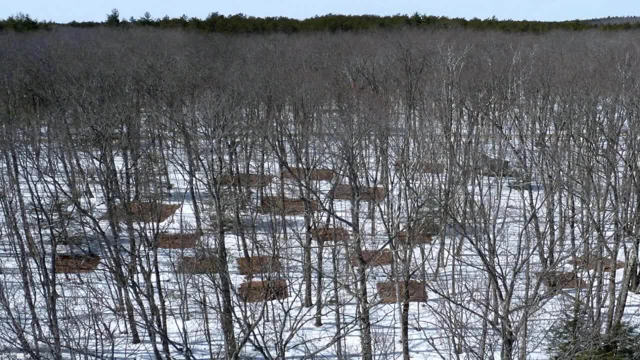 this prospect tail experiment because it's the longest-running experiment. This is a bird's-eye view And you can see the prospect tail experiment in the back. These are six meter by six meter plots And in the front is the swan experiment. the three. 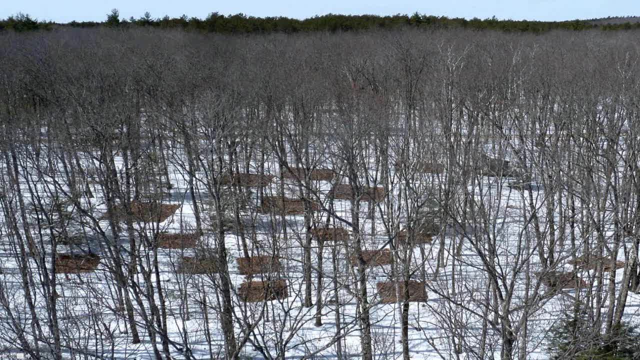 meter by three meter plots. Maybe you can notice this shed. that's our electrical shed, where all the electricity comes in and the data loggers are for controlling the energy to the plots and the thermistors. And here's our access road in the background. This picture was taken from an Eddy flux tower where scientists 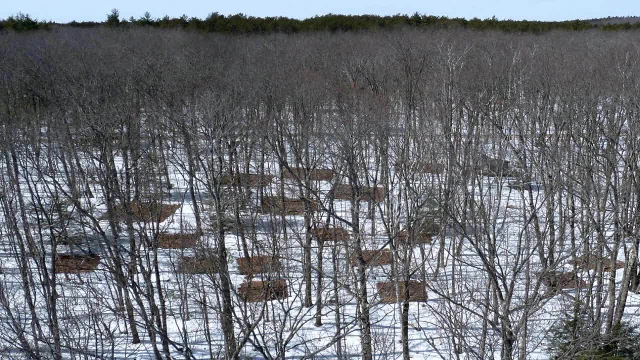 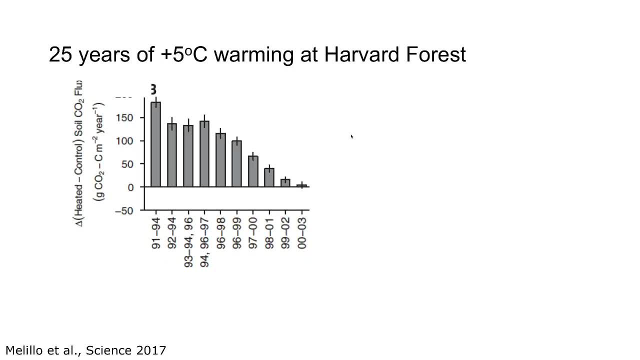 are also studying the atmospheric conditions in the forest and around the world. So what happens when you on heat up the soil in a forest? Well, starting in 1991, now along the x-axis here, this is a three year running average of the difference in the respiration coming. 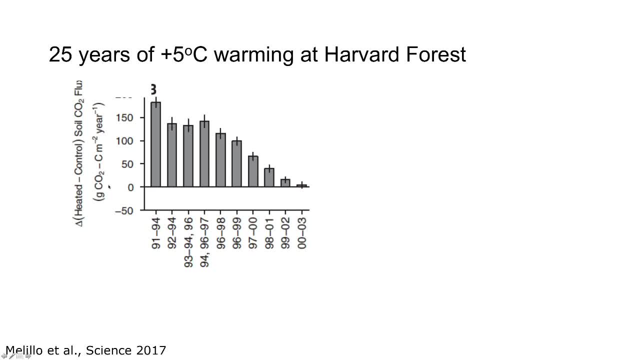 out of the heated versus control. So a zero here would mean that the heated and the control is the same. And so at first, when we heat the system, it really goes faster, and this is just a kinetic effect. You know, you put heat. 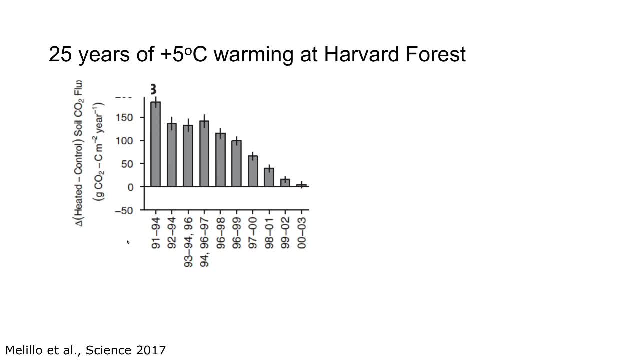 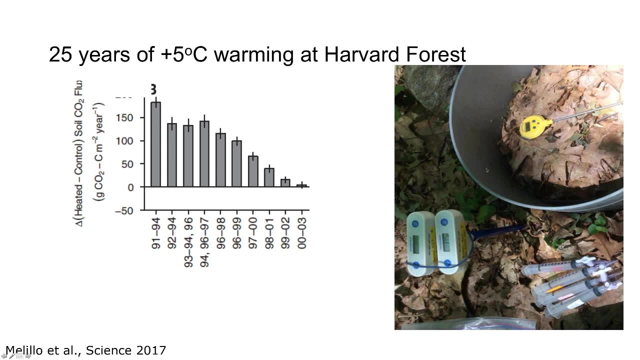 under a kettle of water and the water boils. You heat up the system, the microbes metabolize faster, so they breathe more, But then maybe you can see this decrease in this treatment effect over time, And so the way that we're measuring this is. 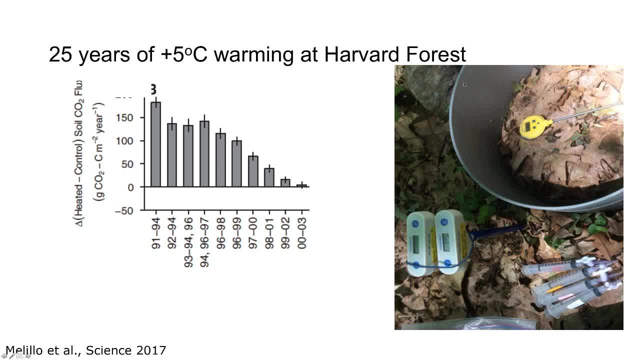 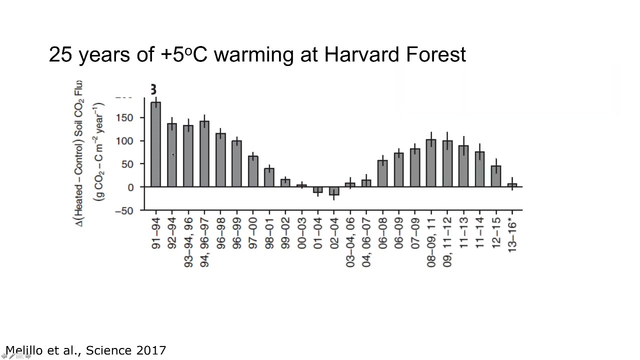 through these cores that are set and permanently installed in the ground. We measure temperature outside, inside, and then use these syringes to collect data from a lid that's collect the CO2 from a lid that's put on, And so what ended up happening is that for the first 10 years or so, there 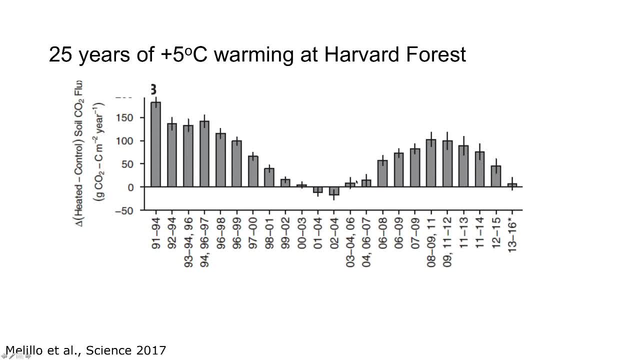 was this kinetic effect, but the effect was lost for a little while. And so what ended up happening is that for the first 10 years or so, there was this kinetic effect, but the effect was lost for a little while and there was no treatment effect. And then it has resumed, And now 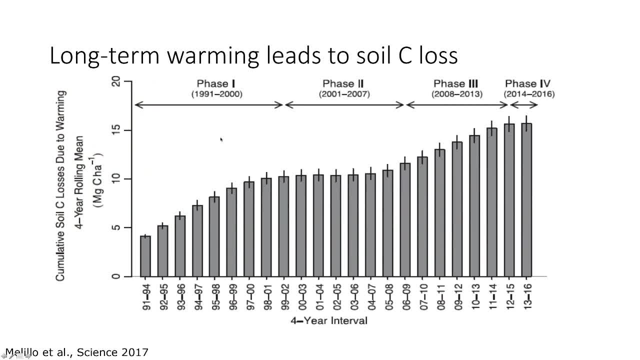 we're looking at maybe even a phase four, And so this is this difference in respiration, And if we look at the carbon loss, you can see that this long-term warming leads to soil carbon loss, but in a punctuated way. So 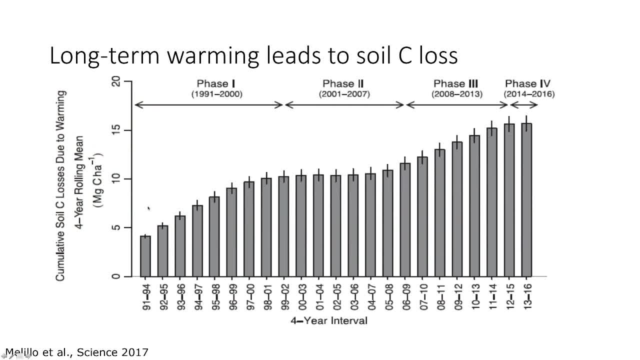 there are periods, like phase one and phase three, of lots of soil carbon loss, punctuated by these intermittent phases where we think that there are changes in the microbial community. And that's where I come in. That's what I'm trying to understand is: how are the microbes changing their behavior to allow more? 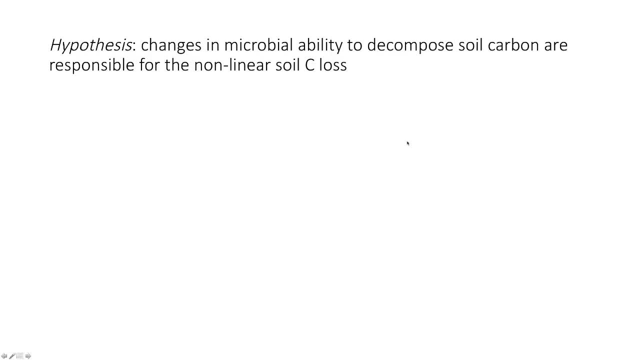 and more carbon to be lost over time. So I'm going to describe to you sort of our process for trying to understand. how is this? what is this non-kinetic effect of warming on soil carbon loss? So our hypothesis coming in was that the 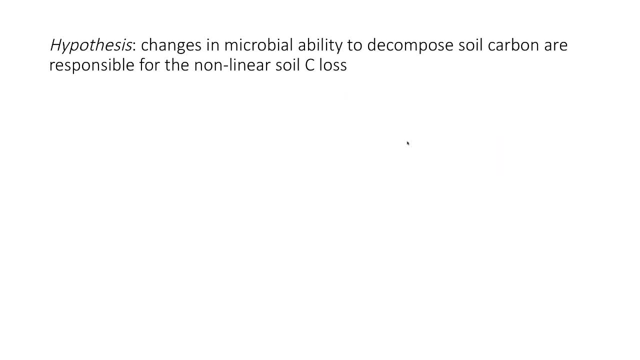 microbes are now better able to decompose soil carbon- two-thirds of their carbon- And so there are changes in the microbial ability to decompose soil carbon And that's why there's this nonlinear soil carbon loss. So, before we begin talking about the scientific 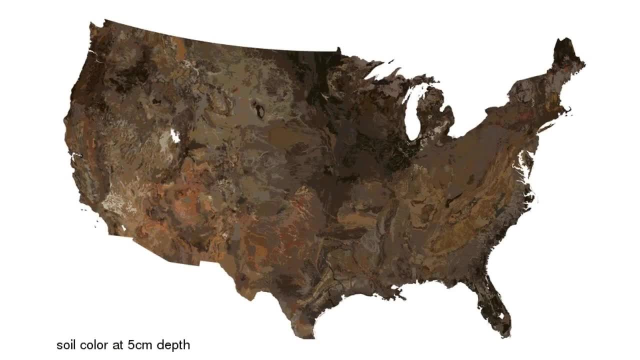 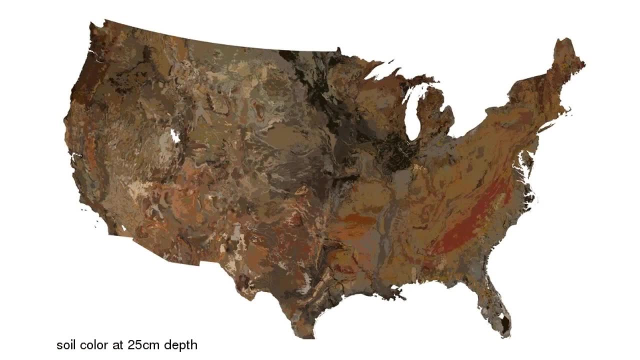 method. I said: you know, when you state a hypothesis, we need to do some investigation first. And I want to talk a little bit about soil. So there's a lot of variability in soil and we're trying to account for this. So this is just a. 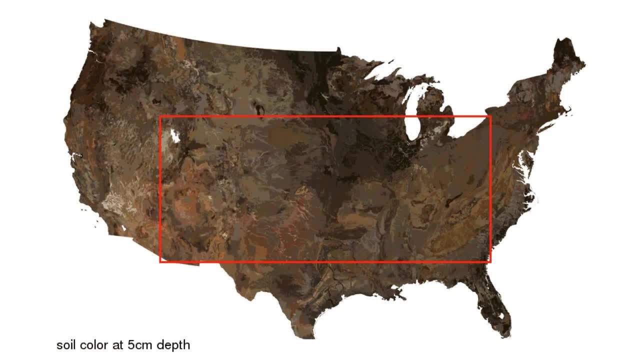 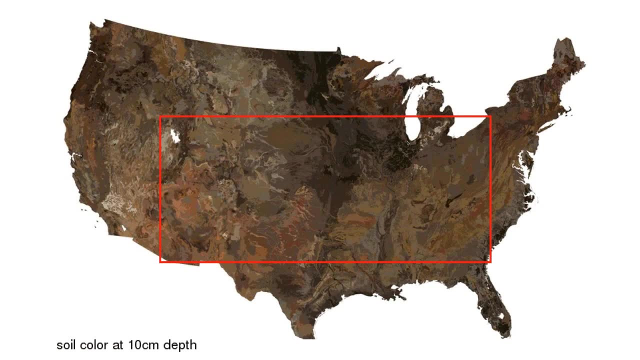 measure of soil color across the United States at five and five and seven inches, 10,, 15, and 25 centimeters depth. So there's some dynamics here, which is partly why we're focusing on one specific system And then, if you focus in 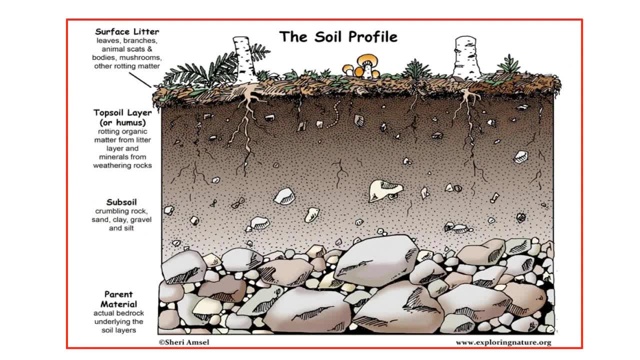 on one specific system. there's also some dynamics in the depth. So at the surface you have a litter layer and then there's an organic horizon soil- in our forest soil Below. that is this mineral layer, and it's this organic horizon mineral layer that I'm going to talk to you about today, And a full soil profile. 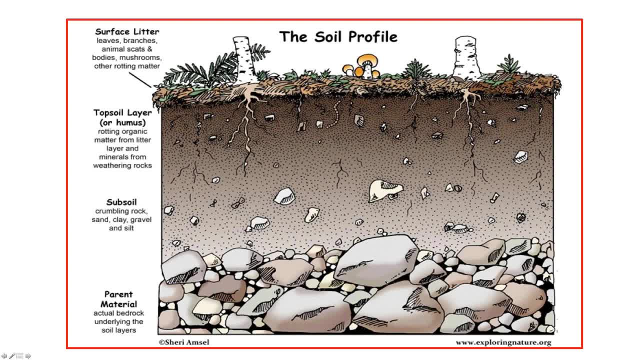 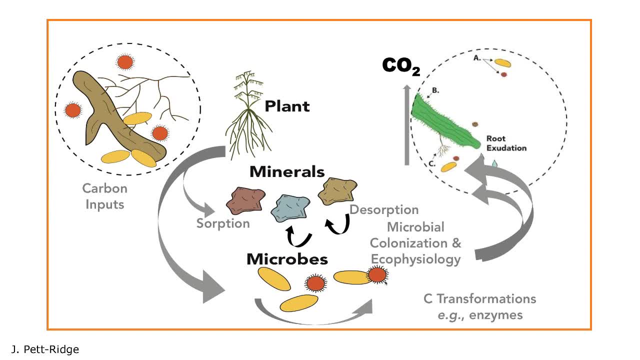 goes right down to the parent material or bedrock at the bottom And then, once we collect our soil samples. what I'm interested in are these microbial interactions, And so if carbon, we're talking about carbon sequestration into soil. so the way that carbon comes into a soil is through plants, through root. 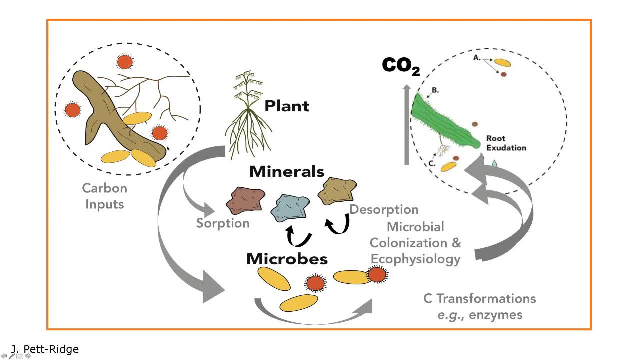 exudates and it can also come in through detritus, So litter or dead root turnover, And that carbon can get sorbed onto minerals. it sticks onto minerals or the microbes can eat it and make more microbes And then through. 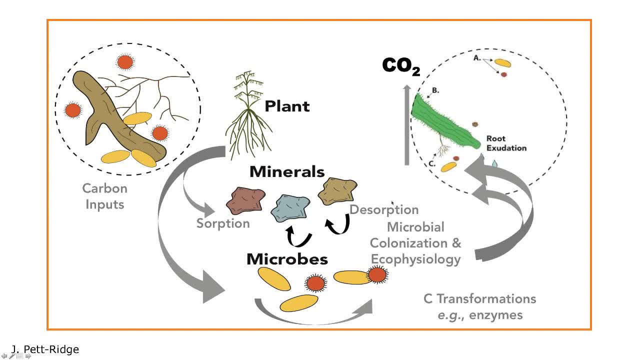 this microbial activity, some of the carbon gets respired and then there is some desorption. that just happens naturally. Part of the way the microbes work is by making enzymes to transform this complex carbon into simple carbon sources that can be eaten. So we have this simple model and I'm adding some 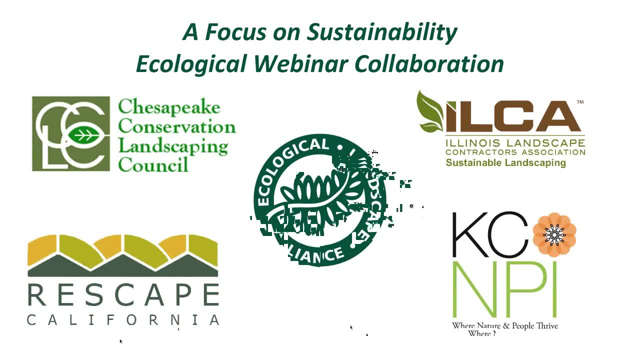 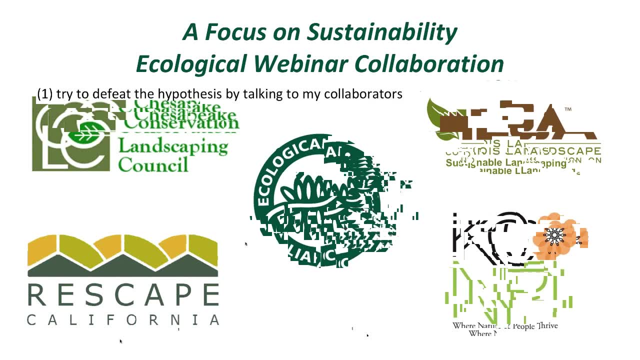 things because these are things that we measure, So we don't have to worry about this too much. but, for example, we can measure the enzymes and measure their rates. So we want to test this hypothesis. The first thing is to try and defeat the 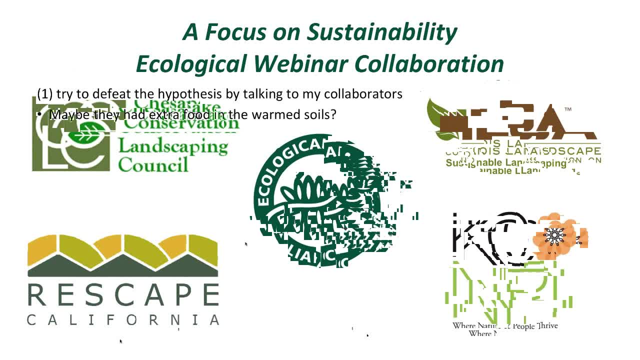 hypothesis. but I don't want to go into the lab just to say, yeah, I want to talk to my collaborators and see what kind of work they have done. So we thought maybe there's more food in the world. maybe there's more food in the world. 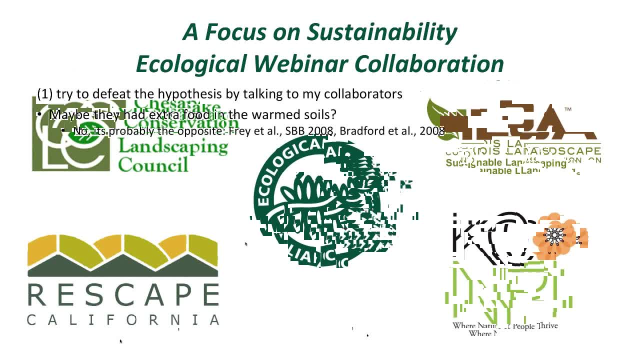 warm soil and that's where the extra carbon is coming from. But no, it's actually probably the opposite. There's less soil, organic matter, in the heated compared to the control. Maybe there were more microbes in the heated and compared to the control and that's why there's this more CO2 coming out. But actually 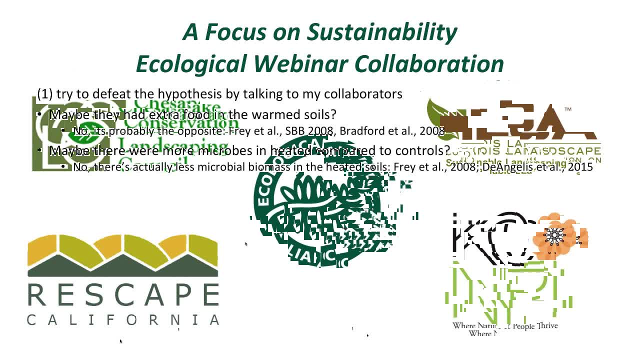 there's less microbial biomass in the heated soils, So that is the opposite of what we would expect. Maybe the microbes were able to adjust to the warmer temperatures somehow, and that's why there's more. But no, there was actually thermal adaptation, but that would have predicted less respiration per unit. 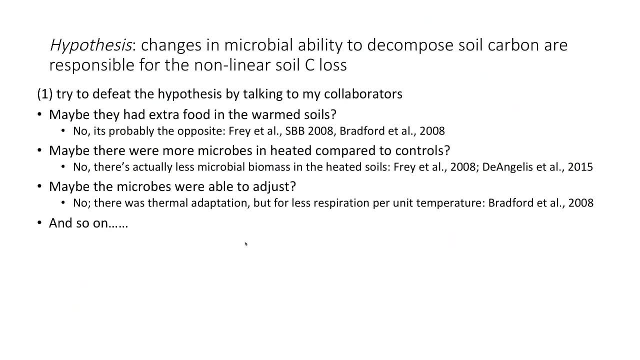 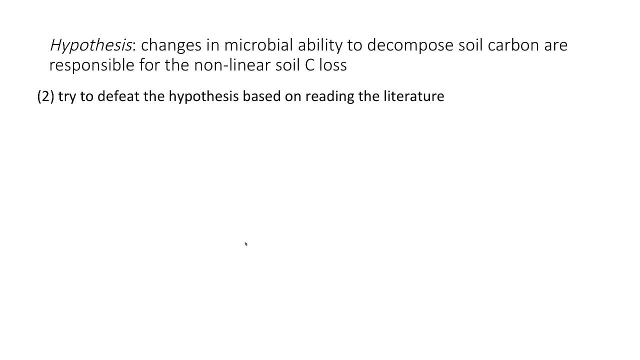 temperature, And so we keep playing this game until I get to a question where someone hasn't asked the question yet. So part of defeating the hypothesis isn't just talking to my collaborators, but reading the literature, And I want to take a moment here to talk to you all about finding peer-reviewed scientific 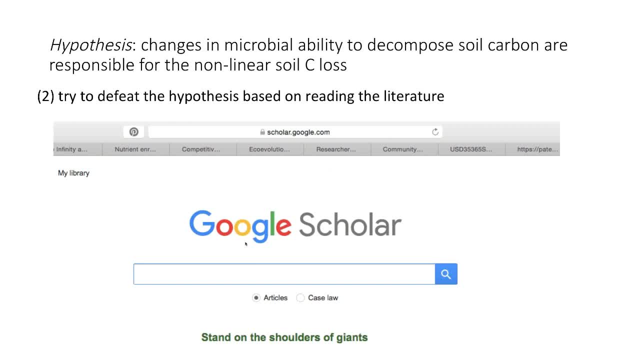 papers on your own. And Guggenheim: I'm sure you've all heard of Guggenheim. Google Scholar is an awesome tool for this And really you can go into Google Scholar and just put in whatever keywords you want and see papers that. 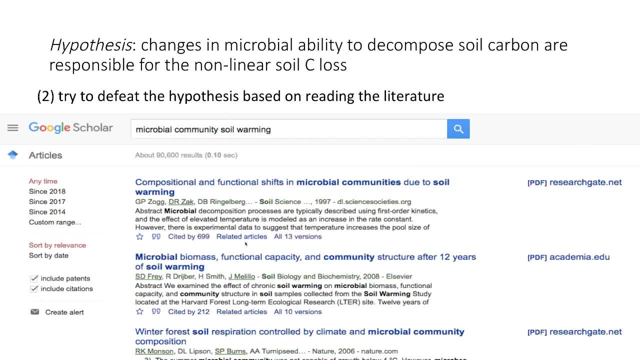 people have found. So, for example, I might look for microbial communities, soil warming papers, And I can narrow this down by recent papers, but the default is that it's going to give me all the papers. There are 90,000 papers that have studied this. somehow They're sorted by relevance And one of the big 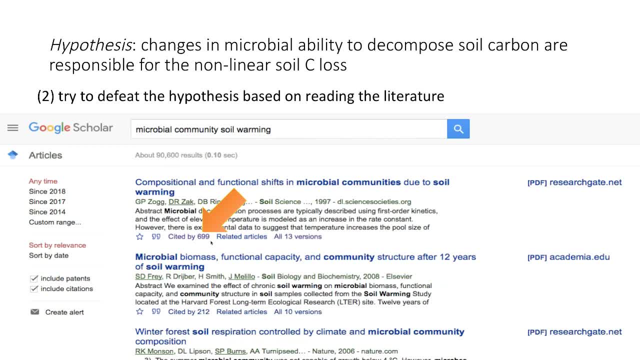 things. if you can see this, this has a lot of citations, So this suggests that a lot of people think that this is a really relevant study for this topic. Now say you were doing this and you really wanted to look at this paper, because 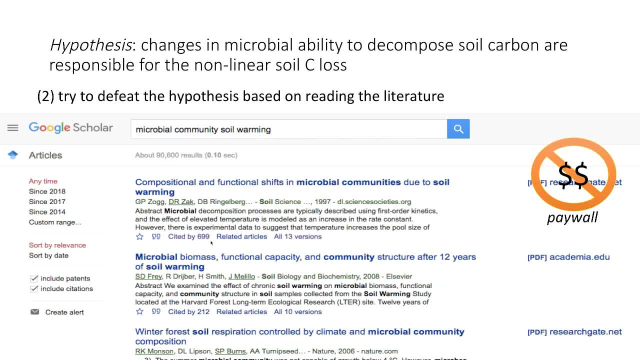 has so many citations but you run into a problem. This PDF link over here there's a paywall. Now, most of the science that scientists do at institutions like UMass and public institutions and researchers does not have any impact on medical research staff. 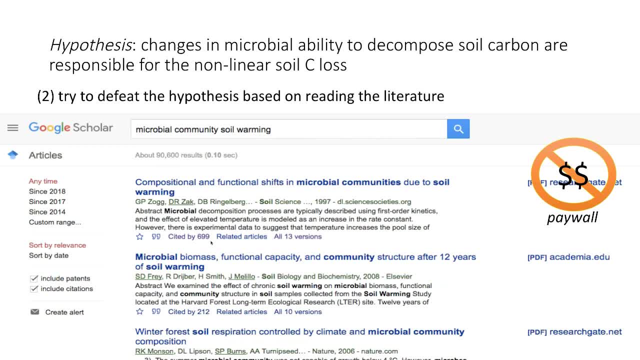 They've gone to research companies like MIT that they've never gone under. They its advised to do research at impossible and grant it, But some of them haven't got a- and government institutions like Department of Energy and the Forest Service. Our research is funded by taxpayers and so it should be open access, and in fact it is, but maybe it's not. 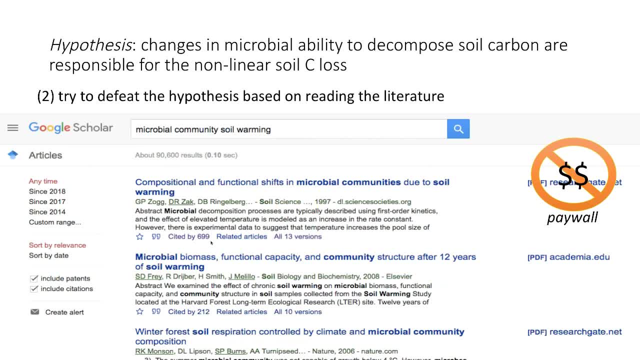 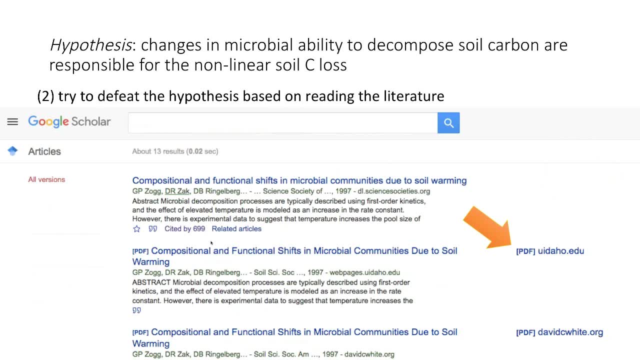 obvious. So here's where you should look. Click this link- all 13 versions- and if you click, look what it is. The University of Idaho has a copy of this paper that you can have for free. It's all, and there are all different places, like here's another one at this foundation website: 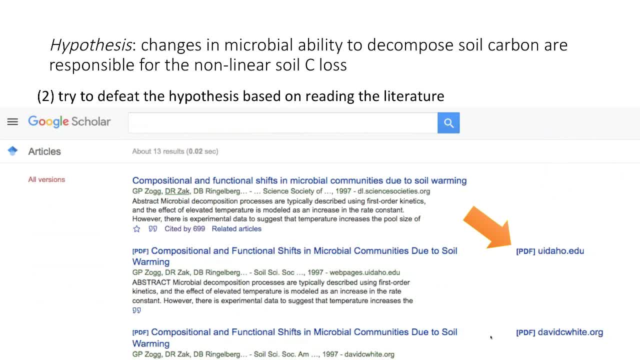 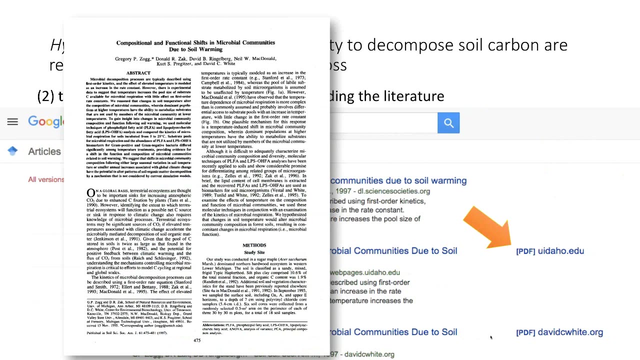 And so you can use this now to get information for your own self on topics that are related to climate change or plant health or some new antibiotic that you're taking and you want to see the medical literature. This is a very powerful tool, And so you click this link and 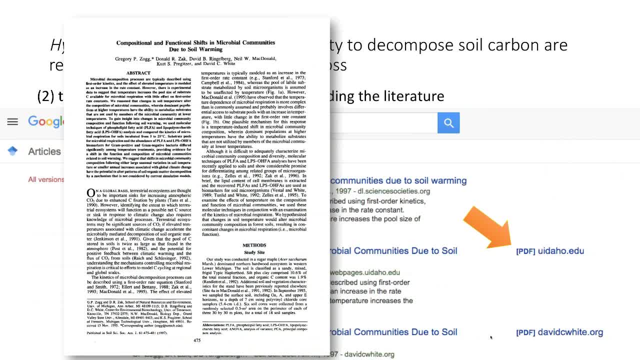 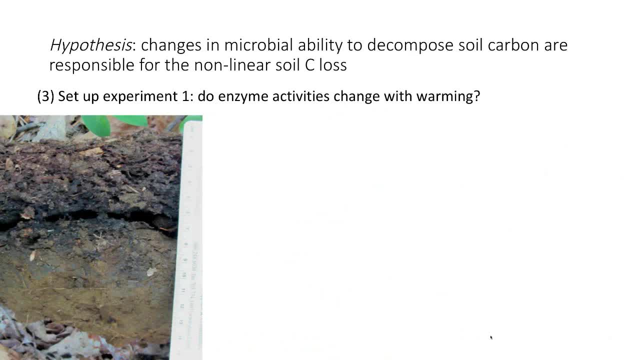 now, here it is the original Zog paper that you can read for your own self at your leisure. Okay, so I've gone through the literature. I'm satisfied that this is my experiment. I want to look at how enzymes work. I want to see how enzymes work. I want to see how enzymes work. I want to see how. 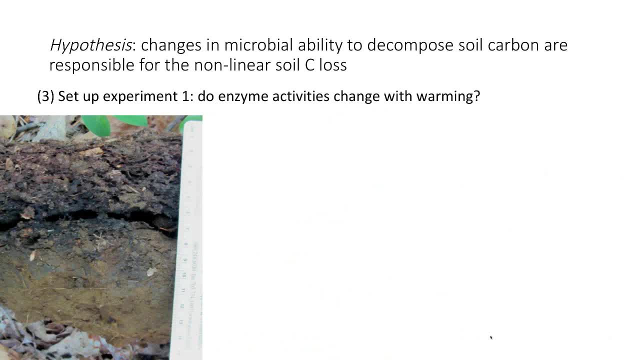 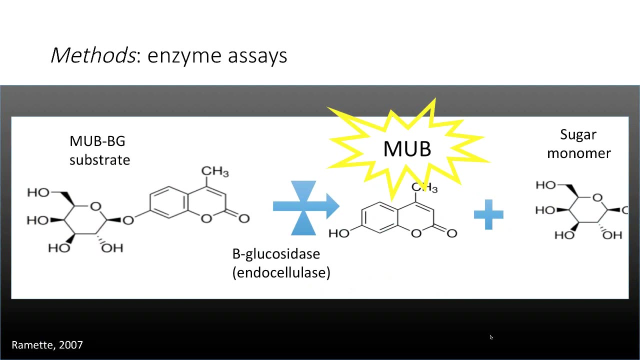 some activities change. Enzymes are decomposing actors, Microbes make enzymes, so maybe they change with warming. And I'm going to focus on these cellulose enzymes, these endocellulases that turn complex cellulose into cellulobiosis, And we have to use an assay. We can't see our 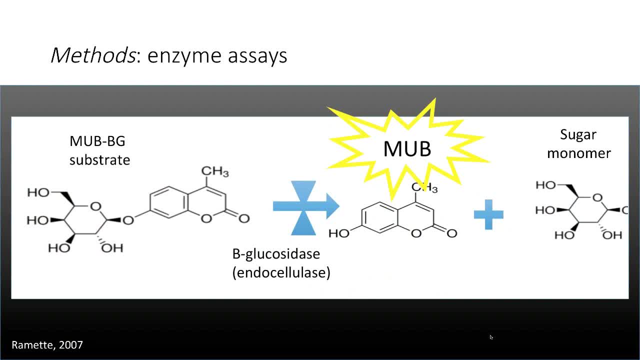 microbes. so we have to have a trick, And so the trick is we feed them this labeled substrate, and half of it looks like cellulose and half of it is this fluorescent molecule, but it's quenched when it's attached to the sugar. This endocellulase breaks this bond. 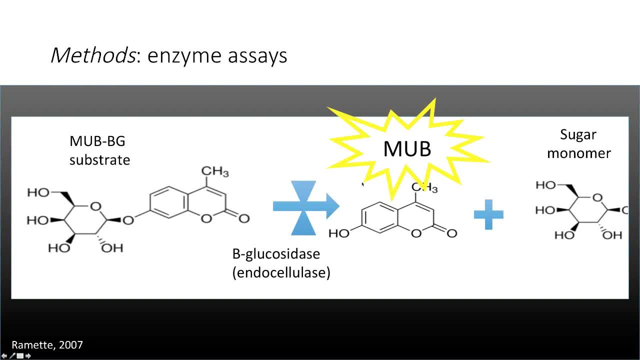 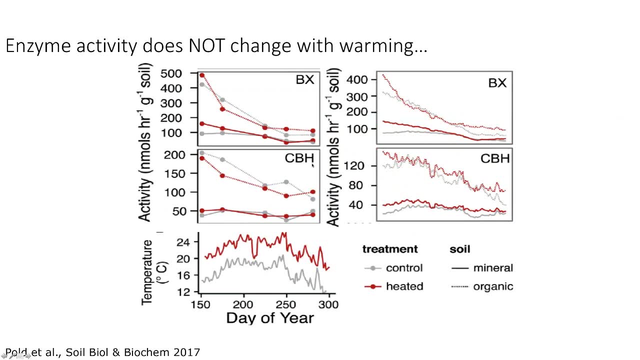 and now this mub is fluorescent and I can measure this fluorescent activity and know what my enzyme activities are for my soils. So this is how we get data like this, where we're looking at enzyme activity And we can see that for the beta-glucosidase enzyme activity, or cello-biohydrolase, 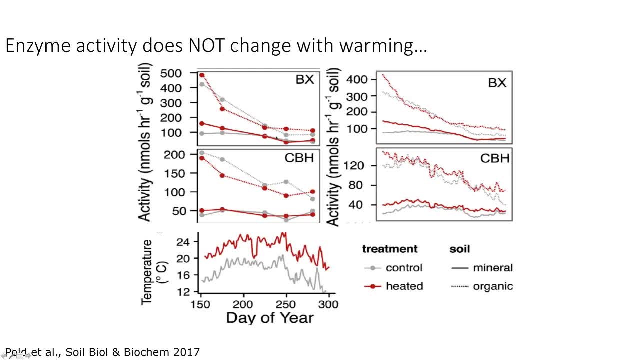 it's not that different on a per gram of soil basis. It's not that different on a per gram of soil basis And even if you look at it, let's see if you correct for temperature based on the actual observed temperature for the day of year. it's not that different. There's a little bit more enzyme. 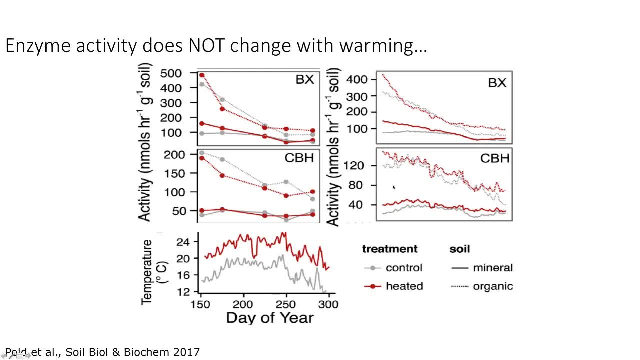 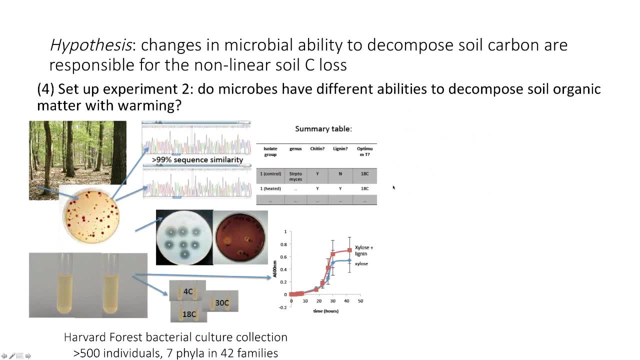 activity in the heated compared to control for this mineral. but it's not a big change. Maybe not a change that would be big enough to account for this big change in respiration. So we're also wanting to look at the microbes that are in the endocellulose enzyme activity. So we're going to 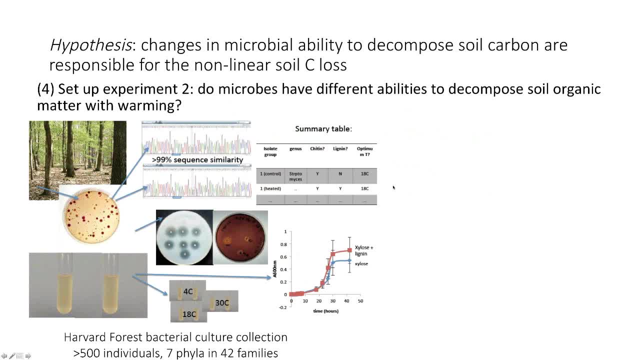 look at the microbes that are in the endocellulose enzyme activity. So we're going to use a lot of microbes to see if microbes have different abilities to decompose soil. So we grow a lot of microbes in our lab And we collect soil from the forest And we inoculate Petri dishes with different types of media. 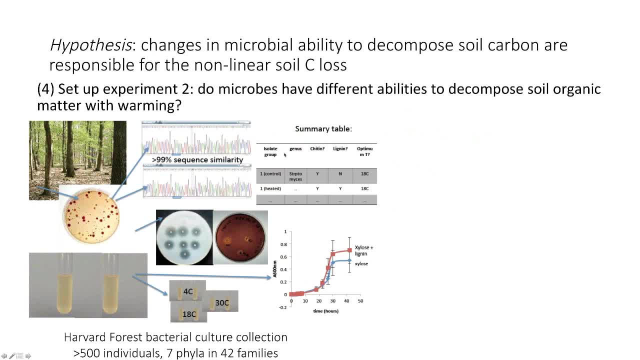 We sequence genes that will allow us to identify what the different organisms are, And then we do tests like: can they grow on different substrates? How do they respond to higher temperatures? Can they grow on complex substrates where maybe you see a zone of clearing for a cellulose plate or a lignin plate? 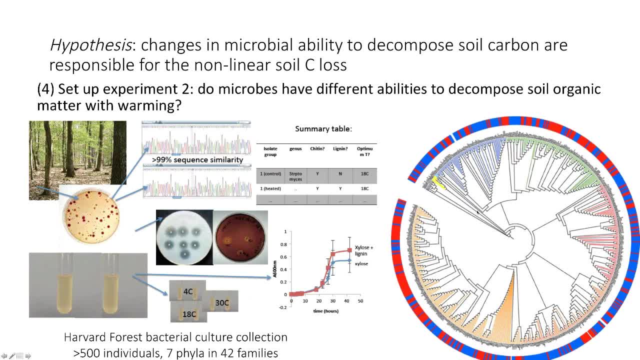 And then we collect him from the forest And then we inoculate Petri dishes with different types of media, We sequence genes, that, And then we can map these traits onto these phylogenetic trees where each branch here is a bacteria and each color bar here shows if the bacteria came from. 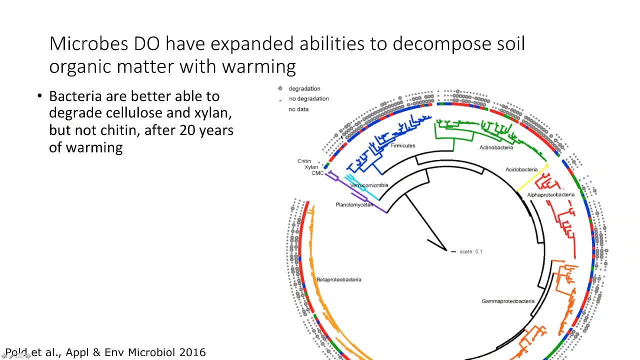 a heated plot or control plot, And what we find if we map these degradation traits onto the bacterial tree is that bacteria actually have gained an ability to degrade cellulose and xylan. that has improved over this 20 years of warming. Chitin, for some reason, was not increased in its degradation. 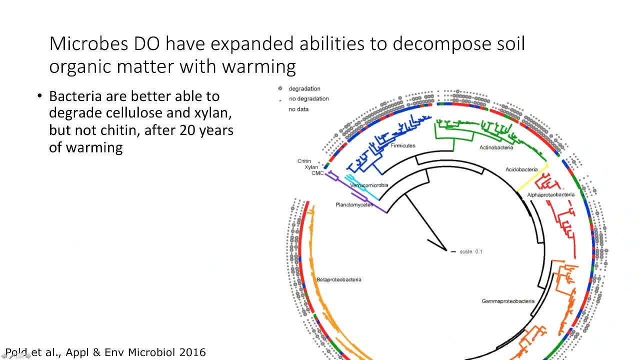 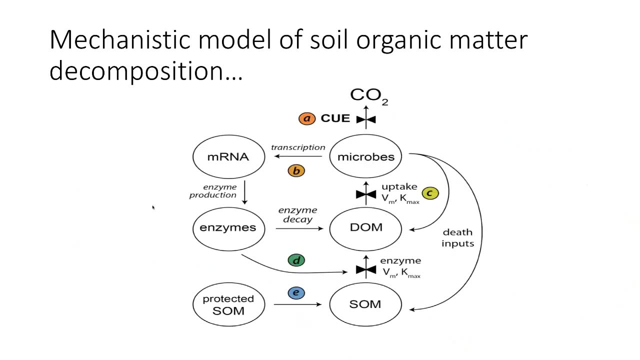 capacity. So bacteria are better able to degrade cellulose and xylan, but have no increased ability for degrading chitin. So this is a way that we can use to show that microbes are decomposing faster and more organic matter with warming. So then, 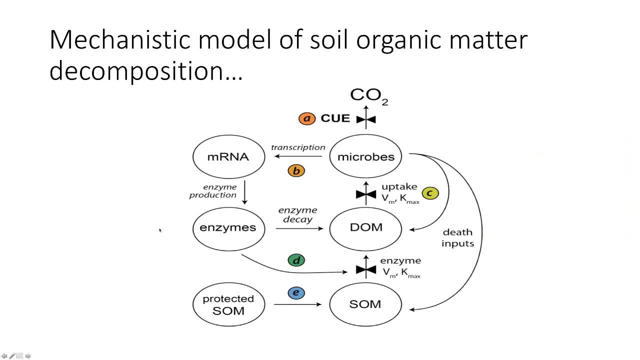 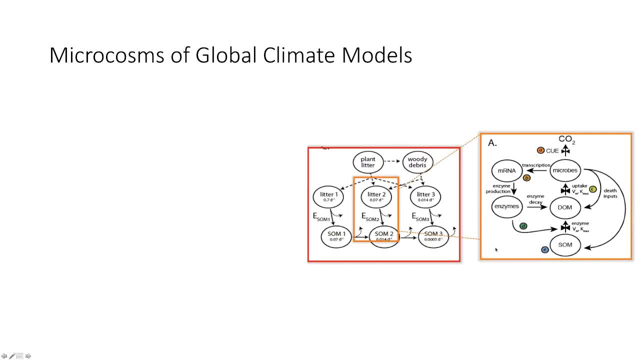 we can update our mechanistic modeling and keep playing this game by sort of testing different things, And so in this way our little model, or little mechanistic model of how things change at this micro scale, can feed in, for example, to this decomposition element of the community land model by maybe informing these different fluxes. 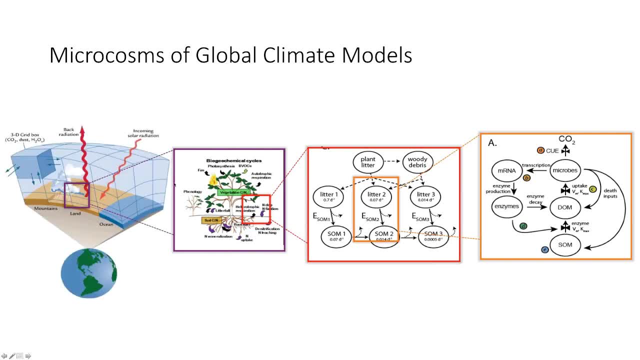 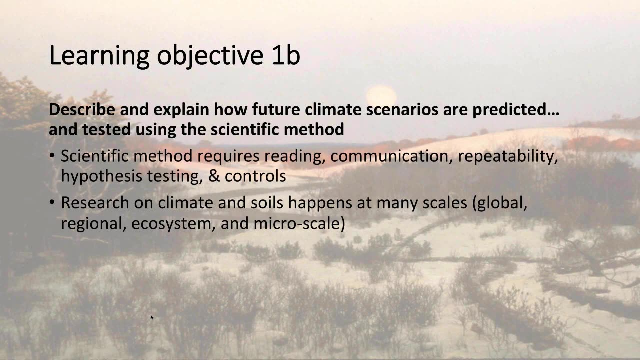 between the litter pools and then that can feed into the big biogeochemistry models, that can then feed into these global models. So that's hopefully just gives you a sense of like how our microbiology can potentially fit into this large-scale. So we talked about the scientific method and how to test. I 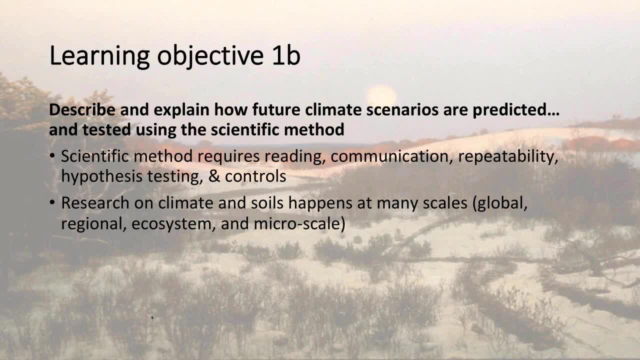 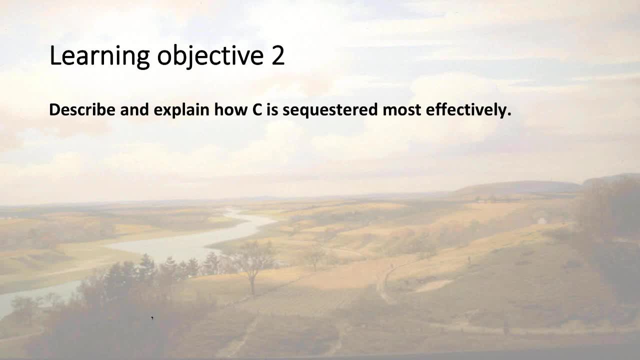 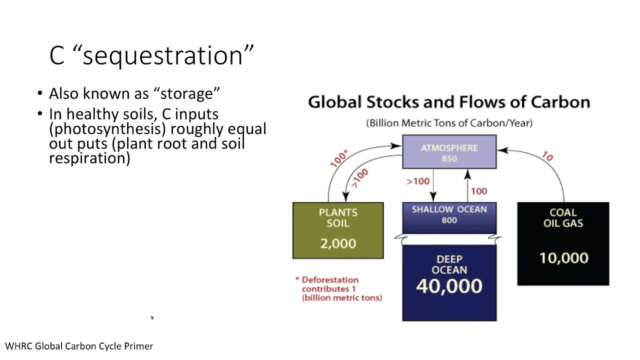 told you a little bit about my own research on climate and soils and how this happens at many scales and our ideas are continuing to evolve. So now I want to talk about how carbon is sequestered most effectively. This idea of carbon sequestration, it's also known as storage. This is another carbon. 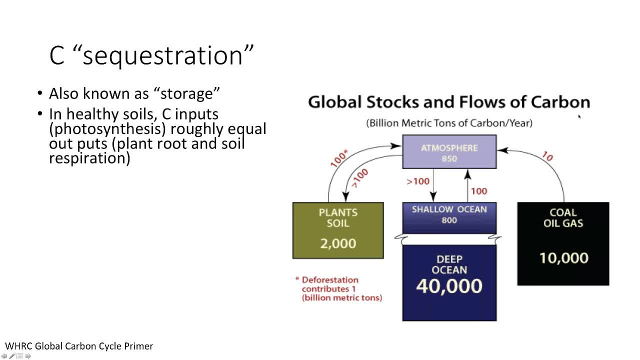 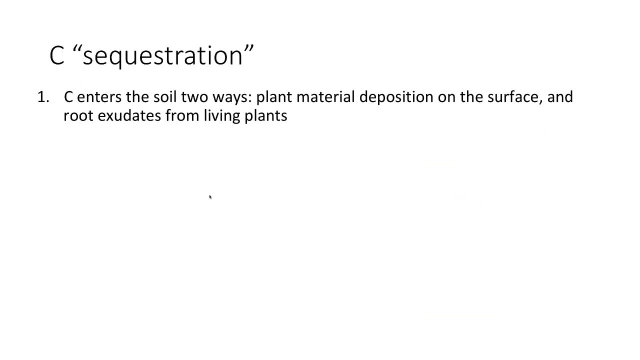 cycle. here's pools, here's fluxes, and this is a global stock, total amount of carbon in the world. And I told you that in healthy soils, carbon inputs roughly equal the outputs, And so carbon enters the soil in two ways: plant. 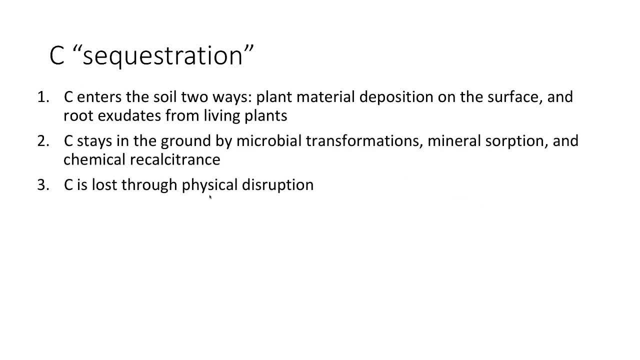 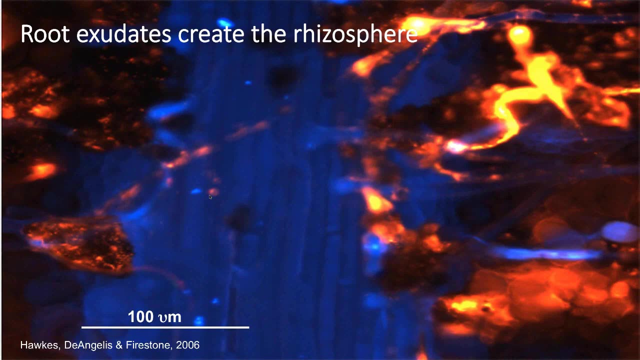 material and root exudates. It stays in the ground by these microbial transformations. One of the ways it can be lost is through physical disruption. So that is digging, tilling, and that's because of this sort of intimate relationship between plants and microbes. So this is a micrograph that I took of 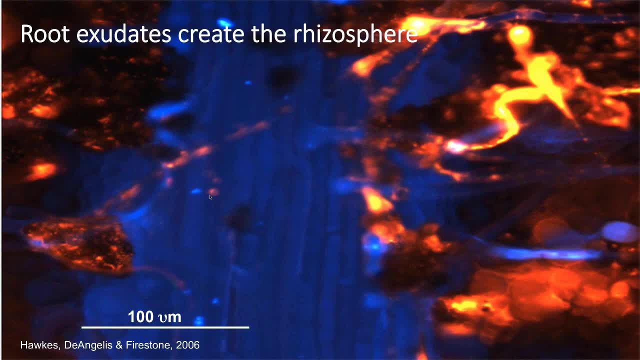 an oat root growing in soil and all of the orange dots are microbes that are living in the soil And root exudates really help to form soil because they create this rhizosphere, they create this environment where microbes can grow and help to store soil carbon. So the rhizosphere, this portion of the 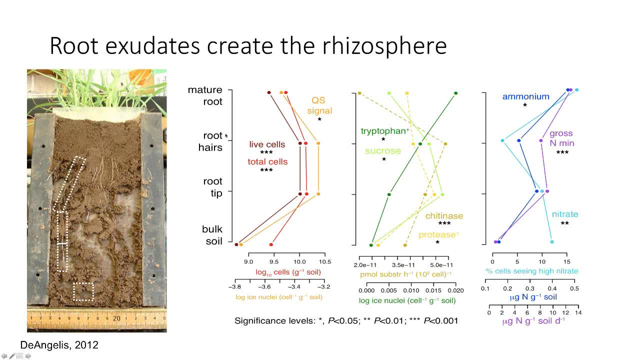 soil that's affected by plant growth. this is a microcosm of the same oat, where we can look at mature roots of this root hair region, root tips and then bulk soil, the soil that's unaffected by roots, and you can see that there's a lot. 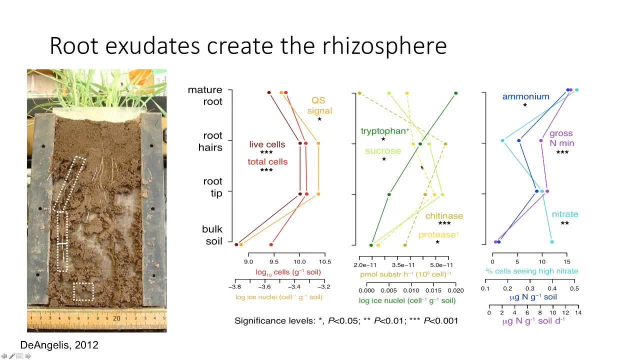 more microbes. they're talking to each other more. there's a lot more sugars, there's a lot more different types of microbes, there's a lot more different Africa, more enzymes and there's a lot more nutrients in the rhizosphere, And this is 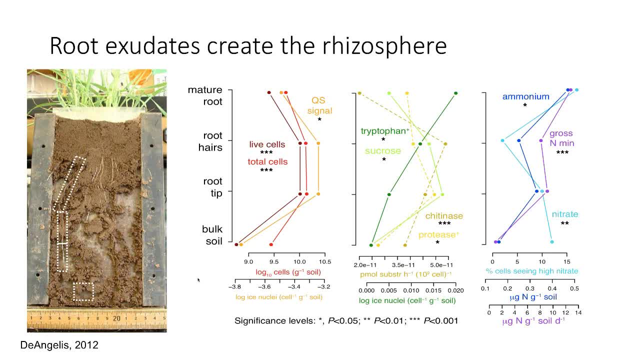 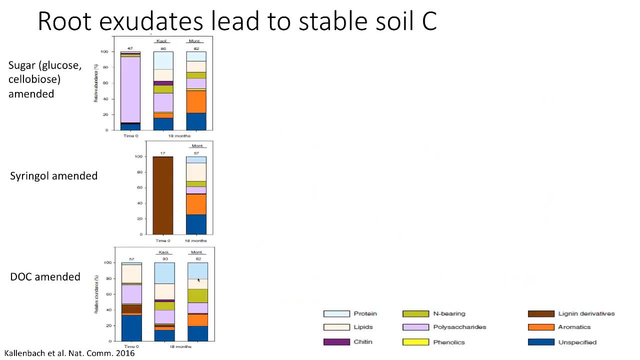 really what this is. the whole point of this plant-microbial interaction is for plants to help microbes so that microbes can help plants with their nutrients. So I told you that root exudates help to form soil carbon and I wanted to show you some data from this paper where the investigators this was: 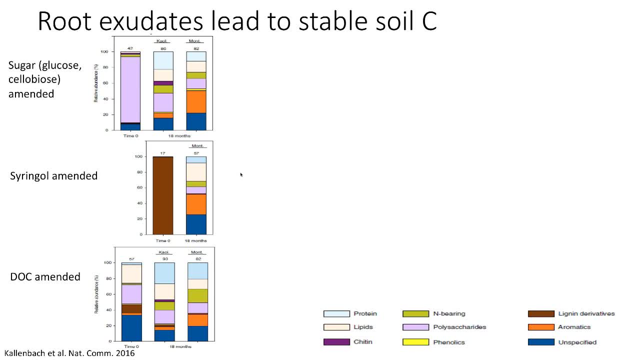 from last year started off with just plain old sand. They inoculated some microbes and then they fed sand and microbes. sugar syringol is a type of lignin monomer or dissolved organic carbon. What they found over the course of almost two years is that, as time goes by, only with microbes and sugar for 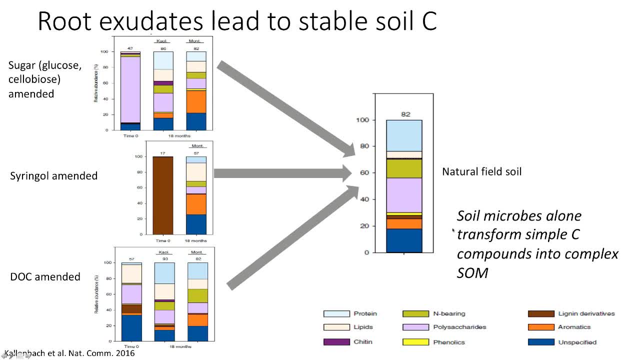 example, the soil carbon chemistry starts to look a lot like the natural field soil. So soil microbes alone are able to transport simple carbon compounds into complex soil organic matter. So this is soil formation happening in the lab, just with microbes and sugar. It's amazing. 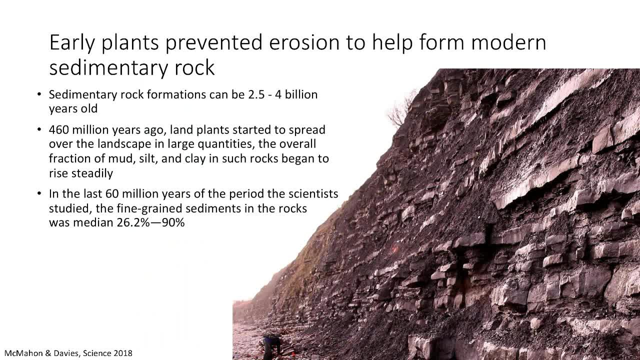 This other study came out last year and this is more of a study looking at rock formations. So sedimentary rock formations can be two and a half to four billion years old. Our planet is something like four point three billion years old. It wasn't until four hundred and sixty million years ago that land plants started to spread over the landscape. 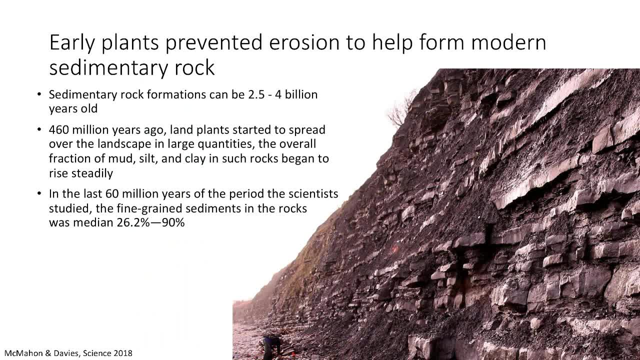 And what these? what the investigators studied was how much of the fine grain sediments in the rocks were in the sediments, And what they found is that it wasn't until plants spread onto the land that they started to have a lot more sediment in the rock- up to 90 percent. 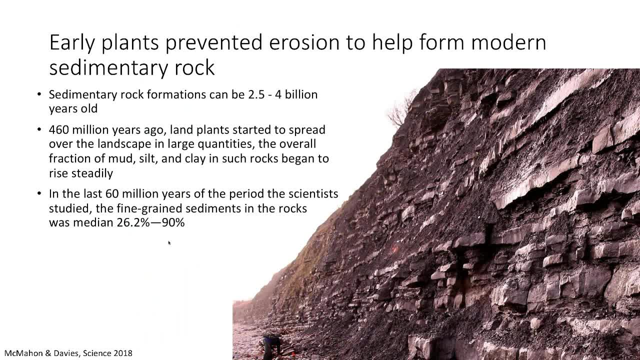 Suggesting that this soil formation was linked to land plants And so these two things are connected, as that early land plants help to form modern sedimentary rock by participating in soil formation. So soils and plants and microbes have been together from the very start. 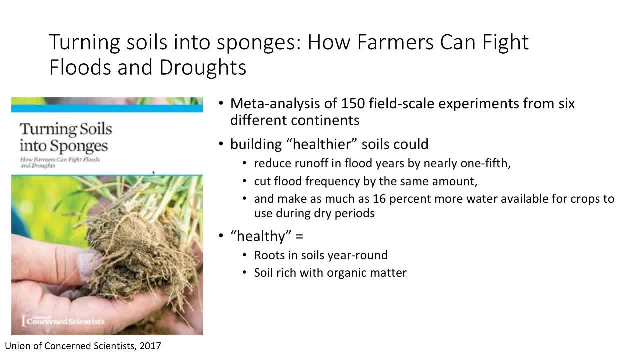 They move out of the bushes that create oxygen and lead over to the land From the very start beginning. So one of the elements of climate change is drought, and we're really interested in what makes a healthy soil and how to keep the carbon in the soil in the face of this potential stress, And so I wanted to tell 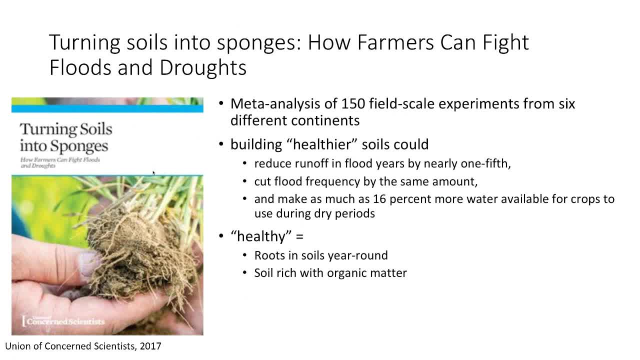 you about the study where they did a meta-analysis. So this is a hundred, and so I just told you about one experiment. This is a an analysis of a hundred and fifty experiments, all from different continents, where they tried to understand what is the effect of drought and how to build healthier. 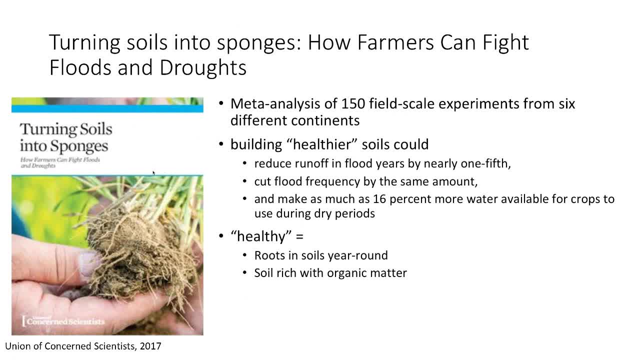 soils, So there's a lot of benefits to having healthier soils reduced runoff, so one of the ways that soil is lost is through erosion. Healthier soils cut flooding frequency by absorbing and acting like a sponge, and they can make as much as 16% more water available. 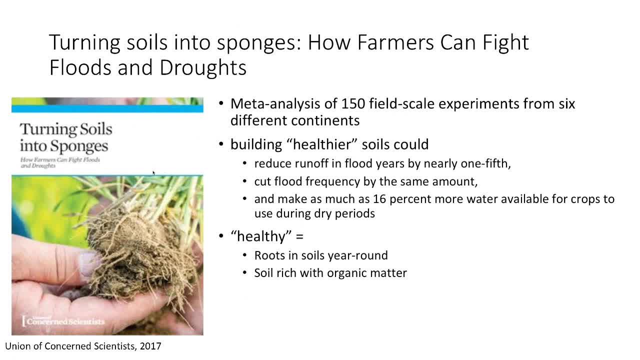 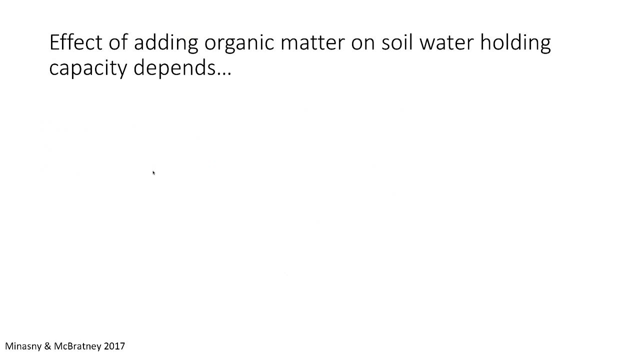 to plants during dry periods. So the this study definition of healthy soils are soils that have roots in soils that are year-round and are rich with organic matter. But maybe you remember when we looked at that map of the United States, of the different soil depths, The amount of added, the effect of adding organic. 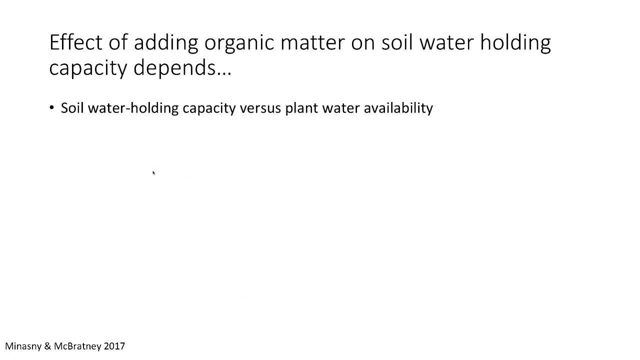 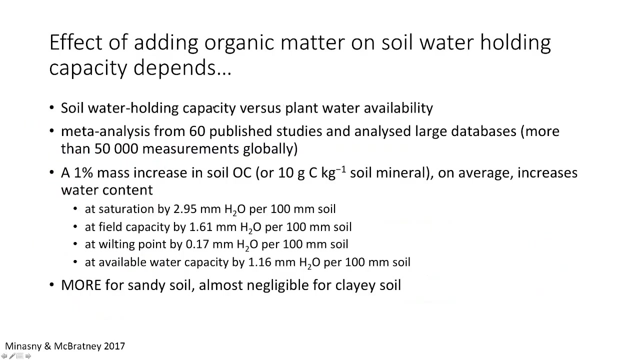 matter really depends. It depends on soil water holding capacity, which can be different than the plant water availability, And so there was a separate study that looked at. 60 is a meta-analysis of 60 published studies. Sorry, my PowerPoint got stuck. Oh, here we go. Let's see. 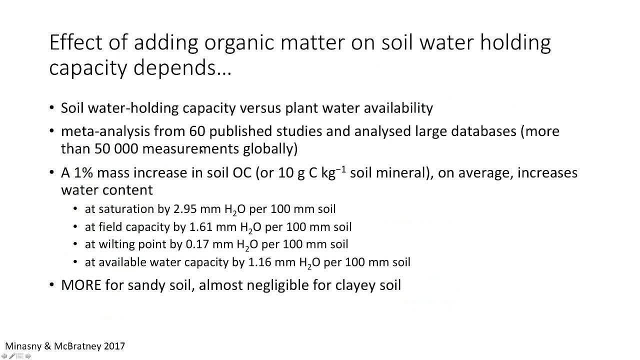 Let's see So of 60 published studies trying to understand how adding organic matter would affect water holding capacity, And the bottom line is that it definitely helps, but it helps more for sandier soils And if you have a really clay soil then adding organic matter it has a very little effect. So it does kind of depend. 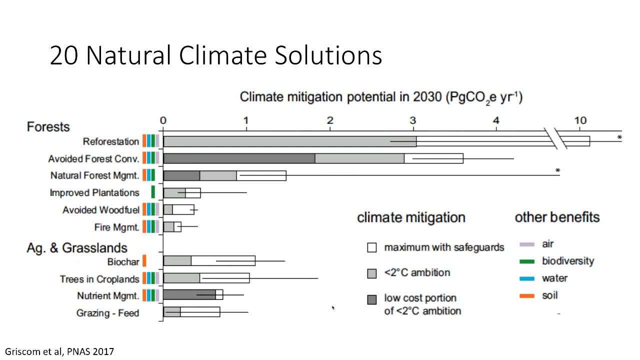 One of the best solutions for natural solutions is having plants in the ground- reforestation, avoiding losing forests. So this is a study where they tried to understand what natural climate solutions would have the most climate mitigation potential by the year 2030. And so this is just a measurement of 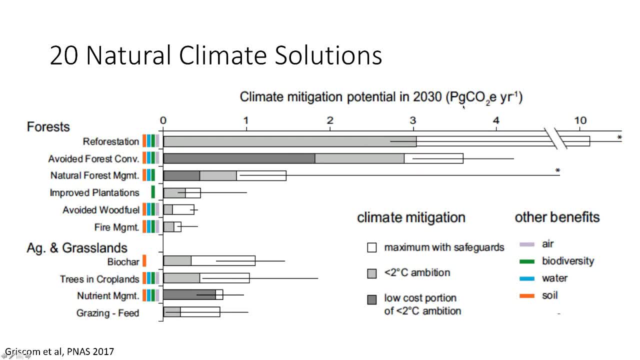 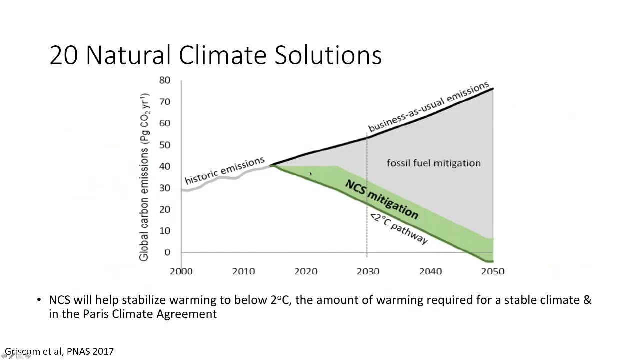 this maximum in terms of the amount of carbon dioxide emitted per year. And what's interesting is if we were to somehow- so I'm just showing you the top- you know eight or nine most impactful natural climate solutions and, like I said, things like reforestation, adding biochar and grasslands- If we did all of 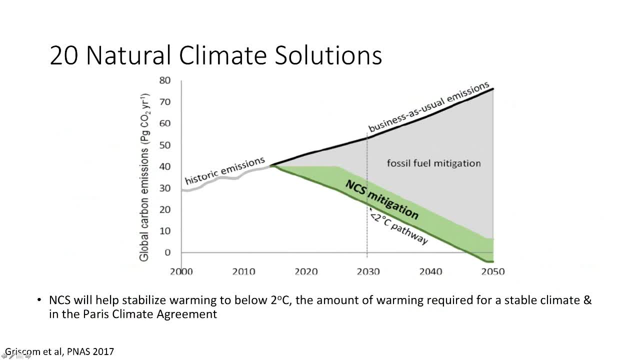 these. it sort of buys us maybe up to ten years for converting our business as usual emissions down to avoiding this two degree global average increased temperature. So this is not a silver bullet, but it helps And this is so. this is something that everyone can do- Most of the soil and 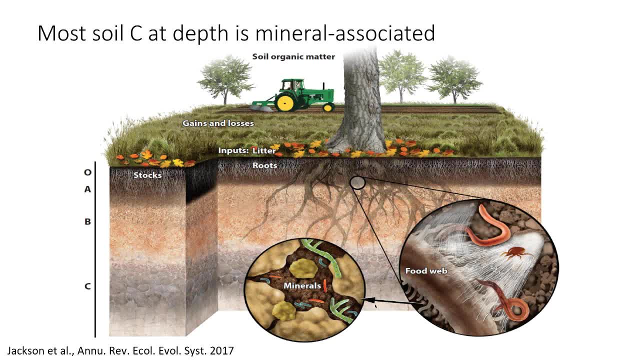 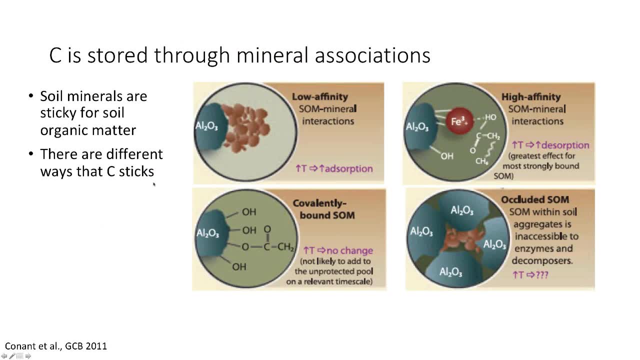 ecosystem is at depth, And so it occurs deep in the ground, well below this rooting zone, And one of the ways that carbon is sorbed in the ground is through these mineral associations. Soil minerals are sticky for organic matter. They can make these low affinity interactions Soil. 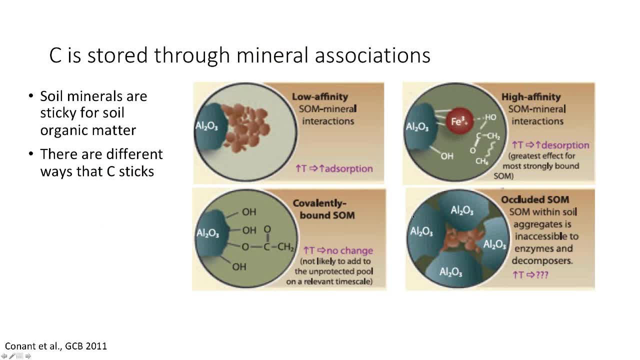 organic matter can be covalently bound through these molecular links. There can be high affinity interactions that are modulated by metals like iron, And it can also be physically occluded in soil aggregates, And so one of the things our lab is doing is trying to understand how these different associations might be. 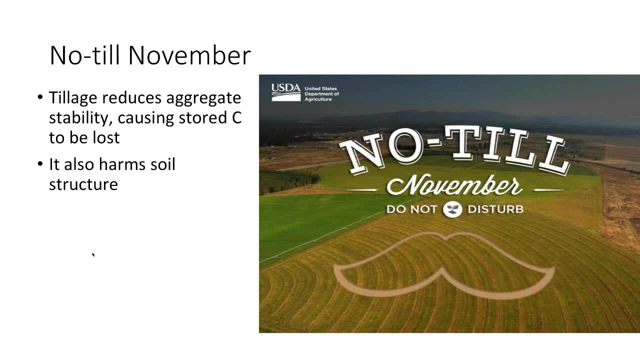 affected by climate change Because physical disruption can disrupt this physical protection of soil carbon. The USDA has started this no till November idea because tillage in agricultural systems reduces aggregate stability and causes the stored soil carbon to be lost. It also harms soil structure. And one thing I didn't put in the slide is one. 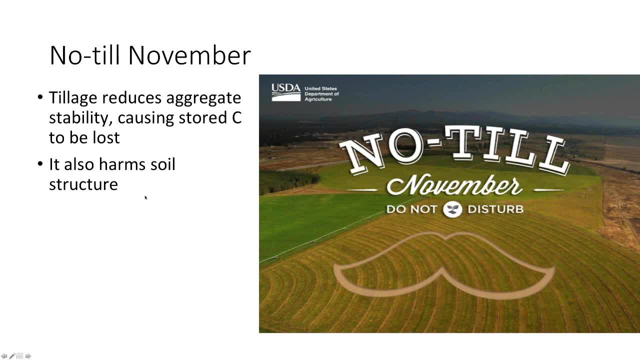 of the problems with harming soil structure is that it breaks up fungal hyphae networks And so the fungi in the soil make these interconnected networks that help to form the structure that are lost. So what? what's a healthy soil? I've been talking about this for a couple of 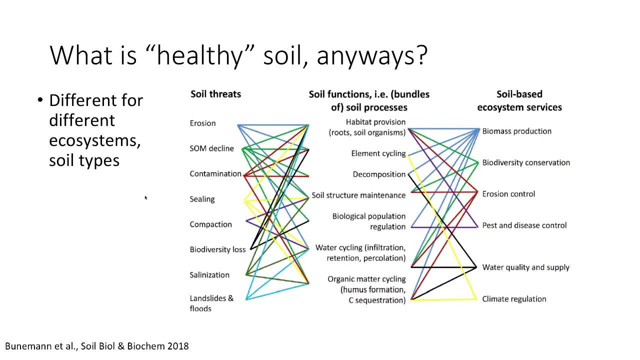 minutes. There are different definitions for different ecosystems and different soil types. This is a recent study from this year where the investigators tried to sort of map out what are different threats, How do we lose soil, What are different functions, What is soil doing And what are soil ecosystem services. 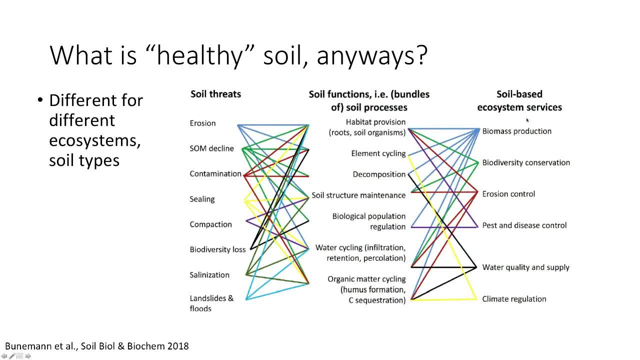 What is coated soil helpful to soil Size? They are becomingって trying to figure out what is a good nitrogen plant that is проблемatize services. What is soil doing for you? It's preventing erosion. it's controlling disease. it's improving your water quality. it's regulating the 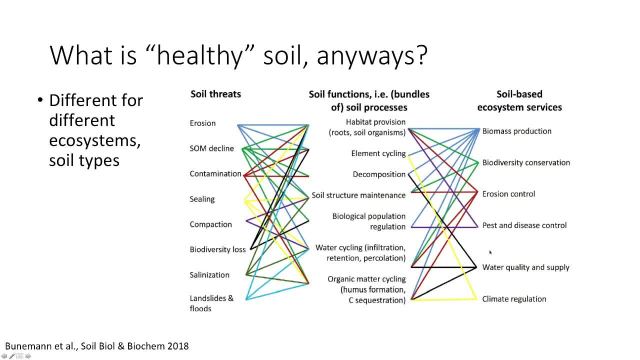 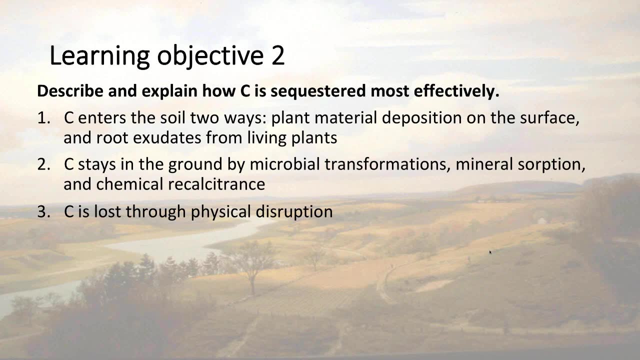 climate And so you know I don't want to go get too into this figure because it's complicated. That's kind of. the point is that the idea of a healthy soil it's a little bit subjective and certainly part of an ongoing study. So we talked about 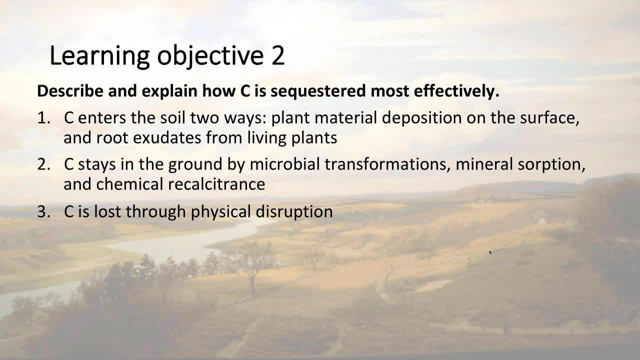 how carbon is sequestered. So carbon enters- sorry carbon enters the soil two ways: through litter deposition and through root exudates from plants, photosynthesizing. It stays in the ground through microbial transformation and mineral sorption, and one of the ways that it's lost is through this physical. 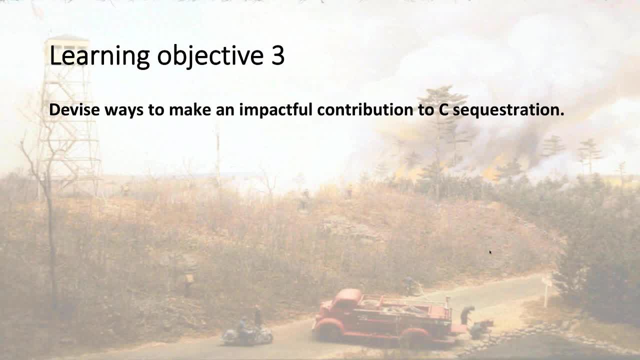 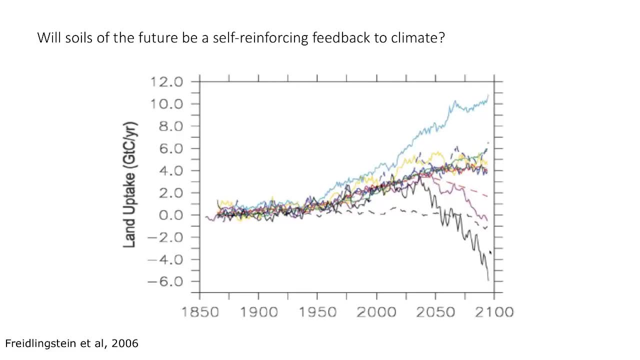 destruction. So we're almost done. I'm gonna finally just talk about some ways to make an impactful contribution as a citizen. You know, one of the things we really interested in is: will soils of the future be a self-reinforcing feedback to climate? And this was a study that was done, a modeling study, in 2006 and the 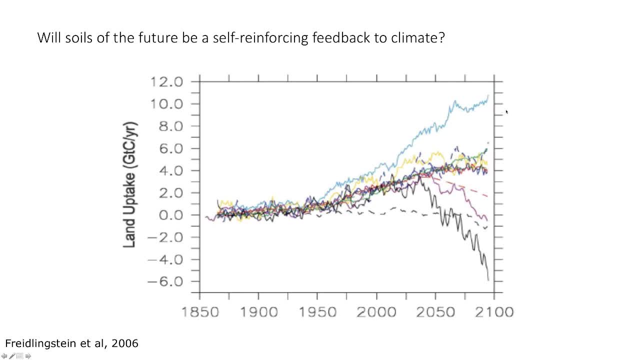 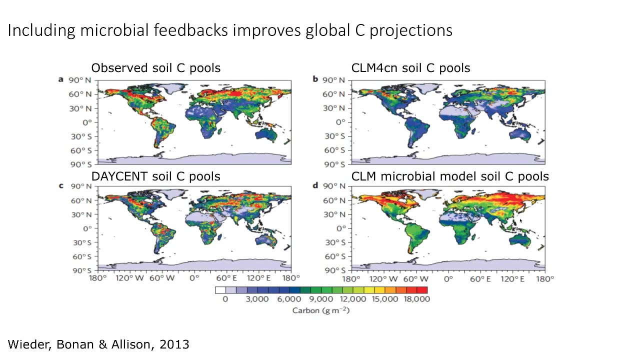 point is, we don't know, Soils could be a self-reinforcing feedback to climate, or they could be a sink, really depending upon what happens. One thing that's clear is that microbes are an integral part of this. So here's a modeling study where 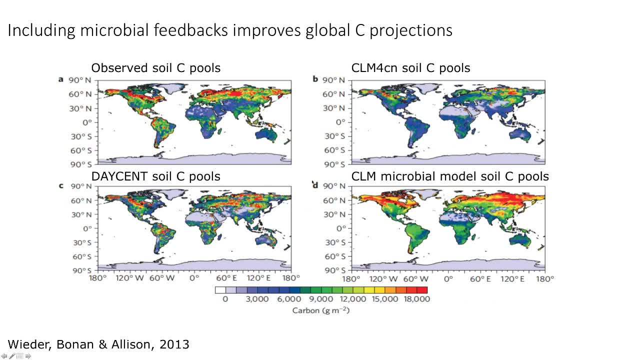 they observe soil carbon pools and then they try to predict them using these different models. So here's a modeling study where they observe soil carbon pools and then they try to predict them using the different models, And what I hope you can see is that in B and C these models don't match. 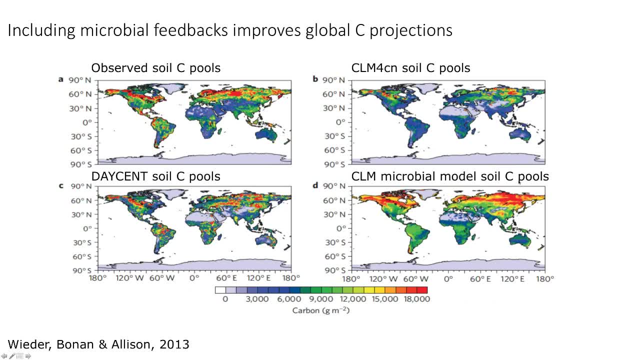 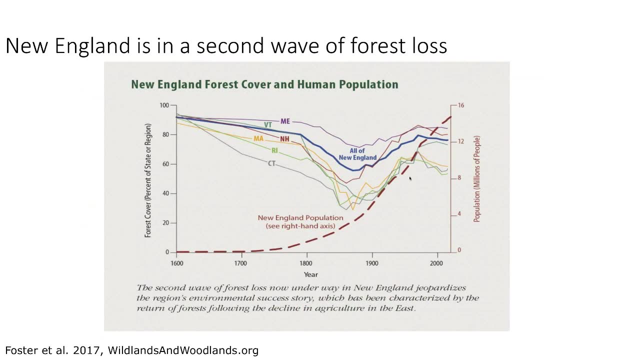 this observed soil carbon pool, as well as the carbon model that incorporates microbes, So microbes are a big part of this soil carbon amounts. Trees certainly are also an important sort of element and, if you didn't know, New England Forest cover is at a new decline. They're calling this the second wave of forest. 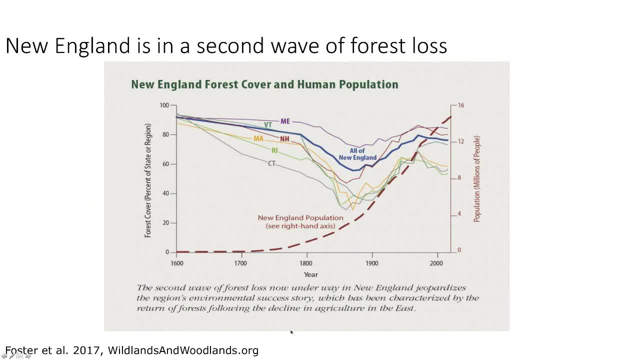 loss and this is part of this Wildlands and Woodlands report that was authored by some investigators of the Harvard Forest last year and the authors are really concerned about this second wave of forest loss because this first wave, which was converting forest into agricultural lands, is reversible and a 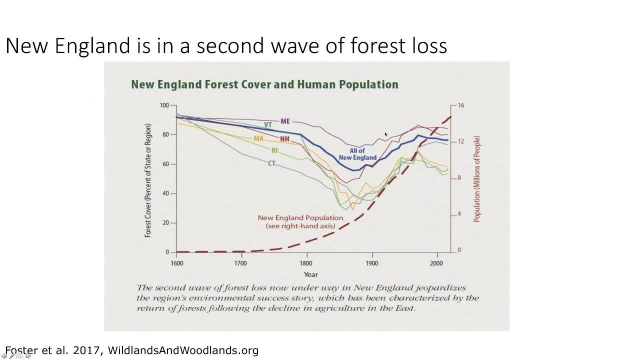 lot of New England recalls later research as a sort of move week after week, where, for example, connected forests became forests are second-generation forests because they grew up after these pastures were abandoned. But this second wave of forest loss now is potentially irreversible because the forests 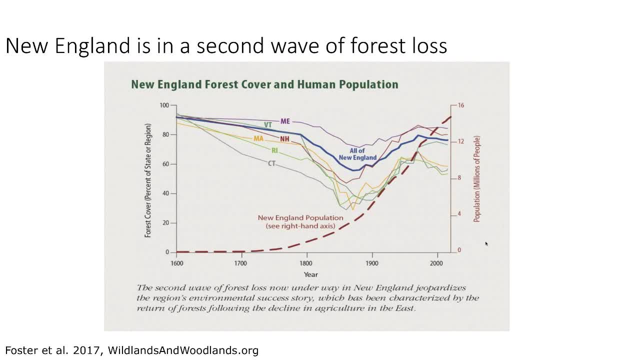 instead of being converted to some other natural systems, are being converted to things like parking lots and developments that are not easily, and in some cases impossible, to reforest over a human timescale. So the National Climate Assessment, then, is a way of understanding. 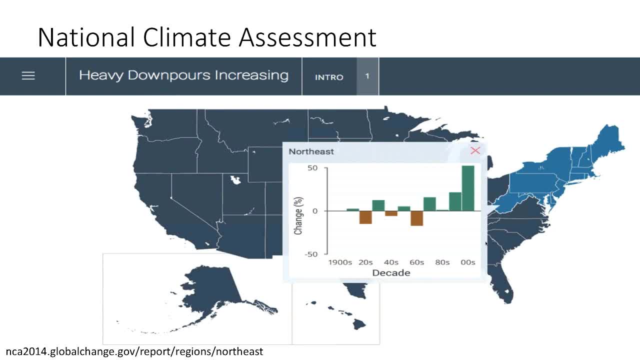 you know for our region or for your specific region, what can you do? And actually New England is one of the regions that the National Climate Assessment is suggesting is a more sensitive region. We in New England are going to feel climate change sooner than our colleagues in 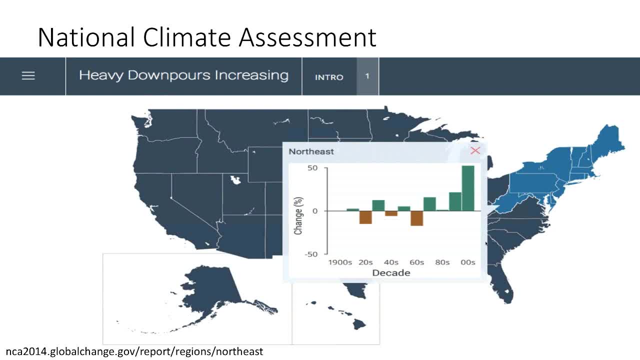 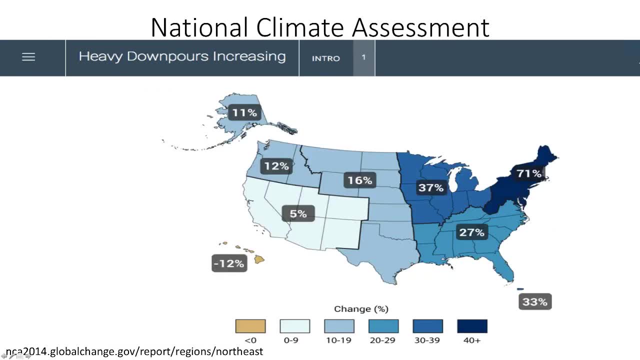 the Midwest, for example, or our friends in the West. So these are the perspectives. These are the percentage changes that we're looking at. For example, heavy downpours are increasing by as much as 71%, And I know that I and all of my neighbors are struggling with. 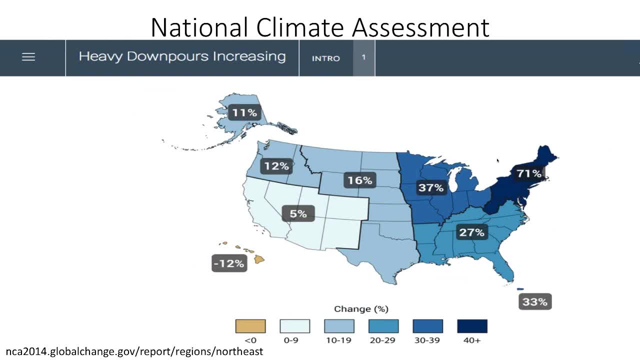 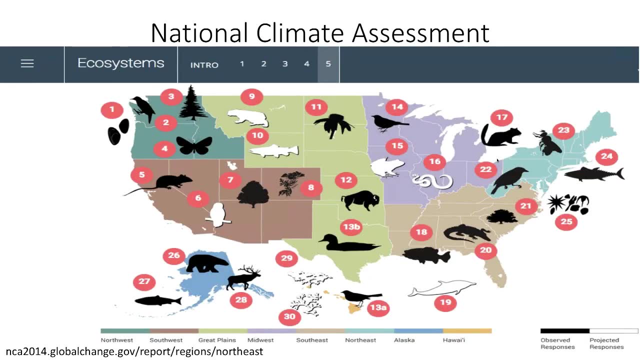 mold problems because it's been so wet this summer. So these are our effects, that were predicted and we're experiencing them right now. So one nice thing that the National Climate Assessment did is it makes some regional recommendations for things, like you know. 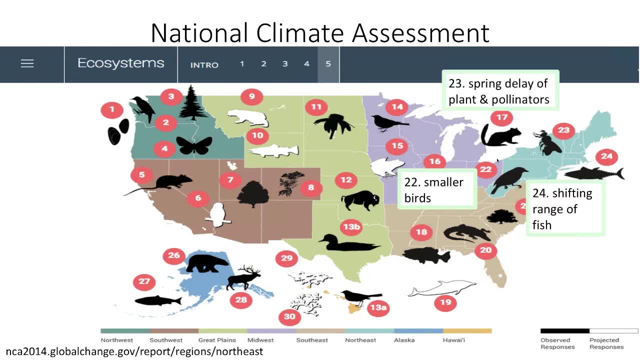 things that you can do to help, And so the New England ones are smaller birds. So if you want to help the birds, you can put out bird feeders. We're seeing a spring delay of plants and pollinators, So plants are blooming later, So the pollinators are coming in later. So if you can, 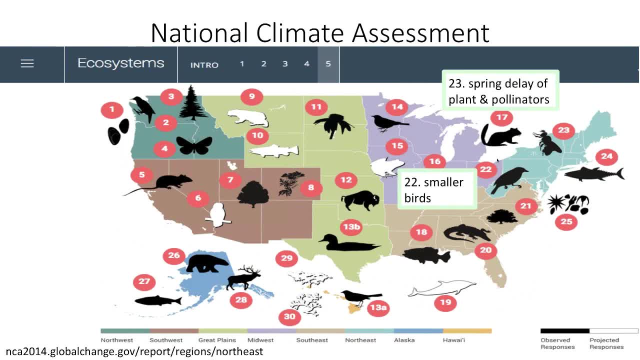 help bees by planting wildflowers. I read recently that you want to have at least 70% native plants on your land in order to encourage pollinators, So it doesn't have to be anything very special, but paying attention to what the local flora should be. And then, finally, 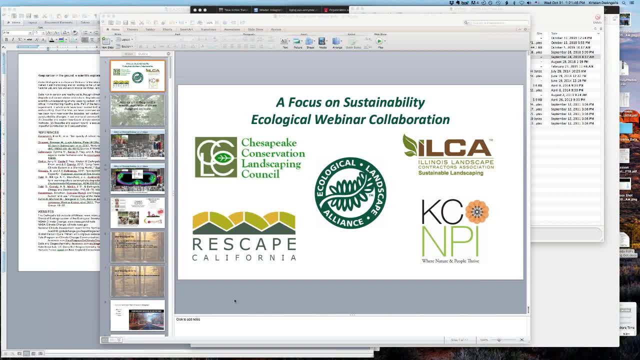 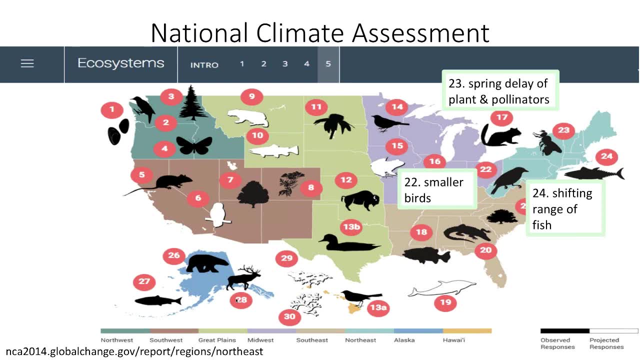 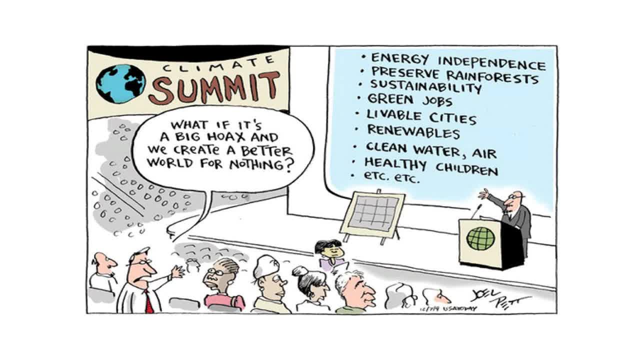 You're going to have to be very careful. You're going to have to be very careful. It's kind of hard for me to understand from where I'm at. I know some people maybe think that it's not real And I'm here to tell you that it's absolutely real. Nobody wants. 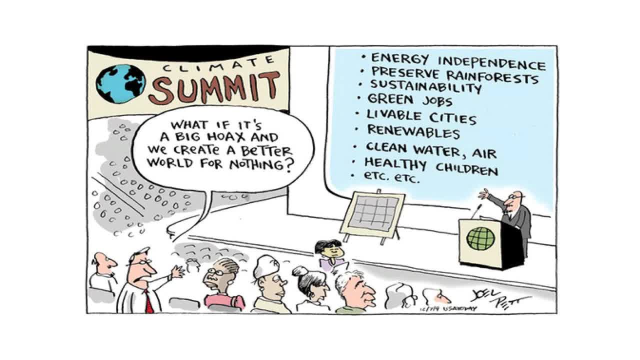 to be wrong more than a climate scientist. But what if it's a big hoax And we create a better world for nothing? I think that this is a win-win situation of you know, keeping plants in the ground, encouraging trees to grow wherever you can, planting trees, making. 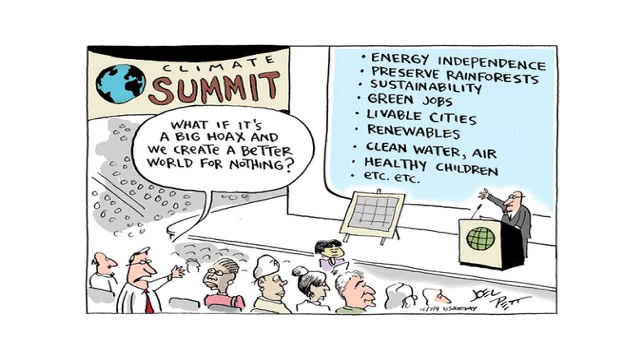 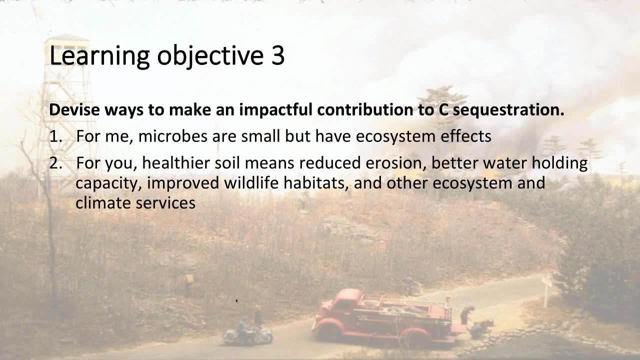 sure you have healthy soil, trying to have as many natives on your property as possible. And then it has all of these other wonderful ancillary effects that just can't go wrong for our communities. So microbes are small but they have big effects And healthier soils. 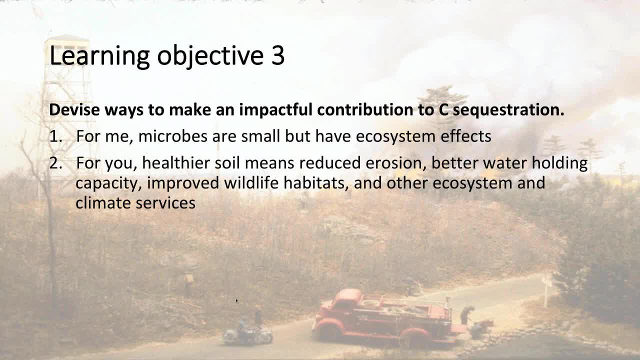 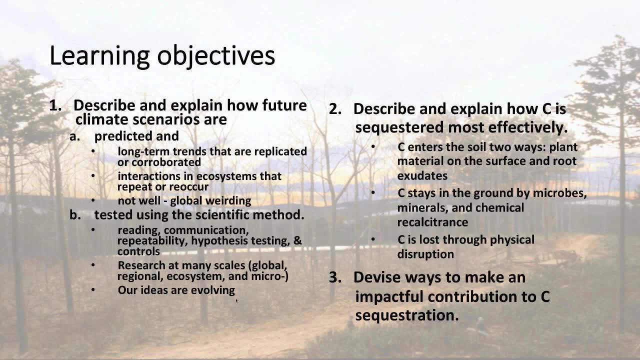 are good for everything: Reduced erosion, better water, more wildlife habitats and many other wonderful services. So this is what I talked about to you today. We talked about how we know about climate change. I talked a little bit about my research and the scientific method. I talked to you. 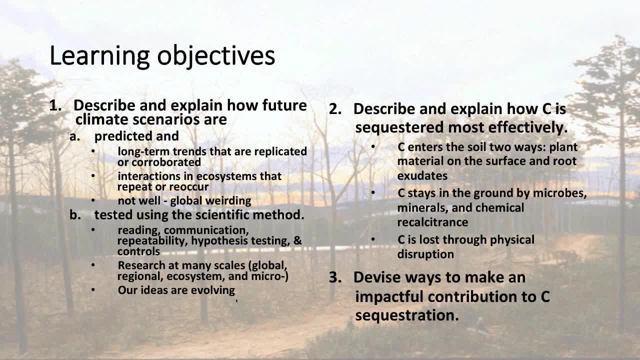 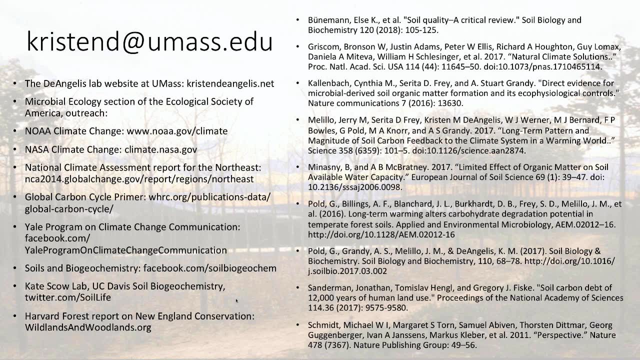 about the ways that carbon can be sequestered, And then I talked about other ways that the folks who wrote this National Climate Assessment suggested. as New Englanders, we can help to make an impactful contribution. And so, for my last slide, I'm going to stop on this kind. 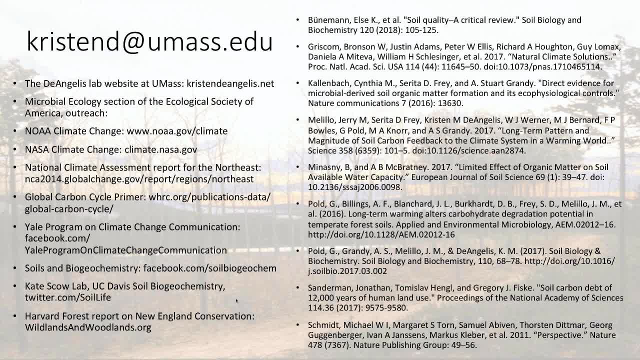 of crazy slide And this is a curated list of references if you wanted to read more about the studies that I showed you. It's not the full list. And then some of the slides and figures that I showed you came from these government websites or these climate change communication websites. 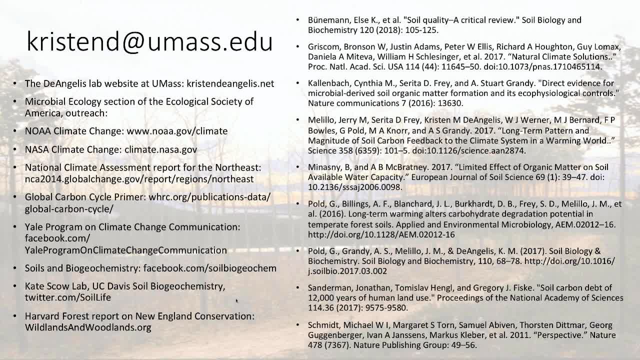 on the left And I definitely encourage you to- you know, don't take my word for it- Go to these different places And learn for yourself about what you can do. And I want to thank you for caring about soil and caring about ecosystems and science. 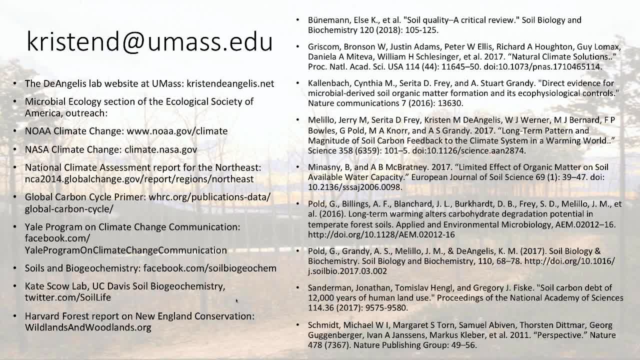 And I'm happy to answer your questions now, And this is my email address And I'm happy to also answer questions over email to the best of my ability. So thanks for reaching out ELA community And hopefully I'll get to talk to some of you soon. 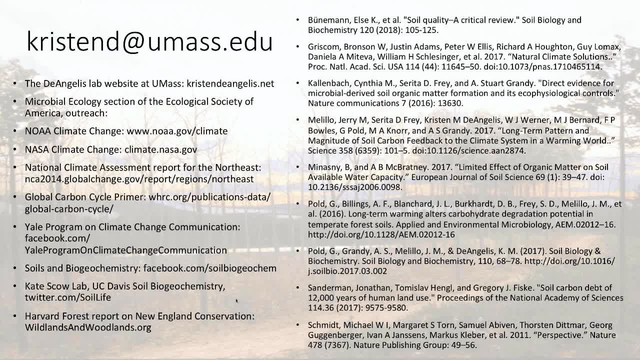 And now I will take some questions, if you have any. Thank you very much, Kristen, And thank you for your patience. while we address the technical difficulties, We have just one question from a listener, And that is why you mentioned toward the end. 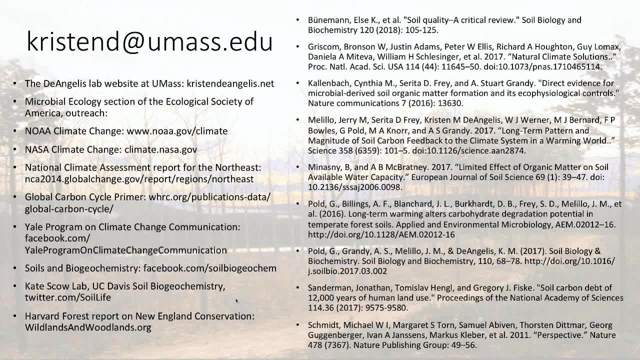 of your presentation that New England will be experiencing more acute climate impacts from the forest loss. Can you explain why that is Well so New England is a region that's expected to experience climate change more acutely than other regions, And that's just because of the way the climate system works. I don't. I'm not sure I can give a better reason for that. It's just that people study and try and understand how the carbon cycle will change with warmer temperatures, different weather patterns And we're expected to warm faster and have more different weather patterns. 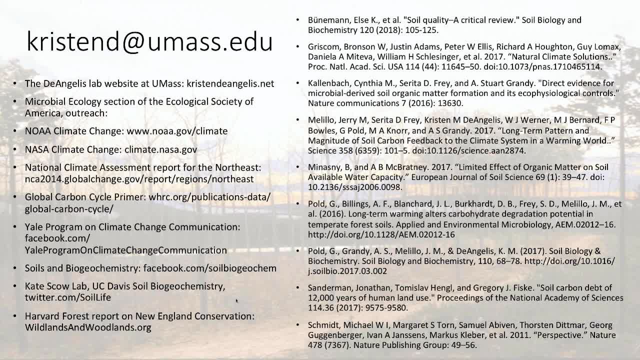 than other places in the country In terms of forest loss. right now we are, as a commonwealth, doing a lot of unsustainable development, So privatizing forests of people who are turning them into, I don't know- parking lots and strip malls. 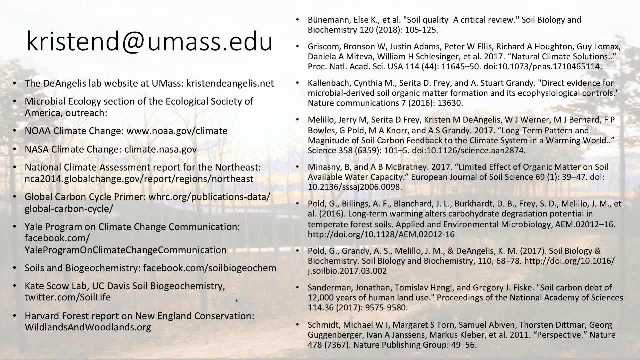 and things like that, and and all I'm saying is we're collecting this data and we're losing forests at a rate that we can measure at this, this regional scale, and once you convert a forest into a strip mall, it is practically impossible to turn it back into a forest. so my point is just that forests provide. 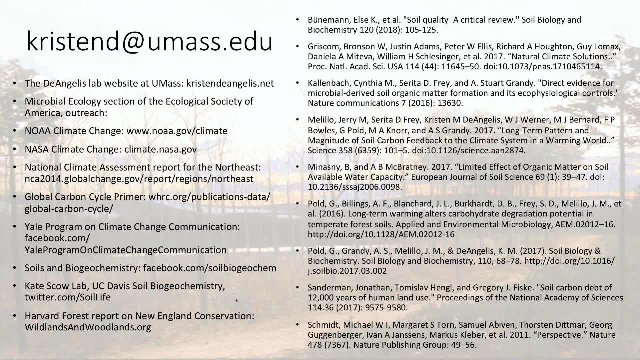 ecosystem services by storing carbon in trees, storing carbon in the ground, cleaning our air and water and that. so these two things are definitely kind of connected. I hope that answers the question. thank you, yeah. the next question is: what role do you feel meadow style plantings have and can have in? 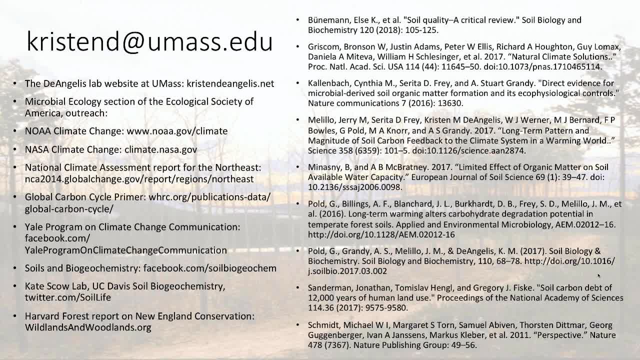 contrast with forest plantings and retaining soil carbon. oh yeah, awesome question. you know I focus on forests because that's what I study, but meadows are absolutely important and I know that there are a lot of like natural meadow communities around and you know, one of the sort of natural succession is from 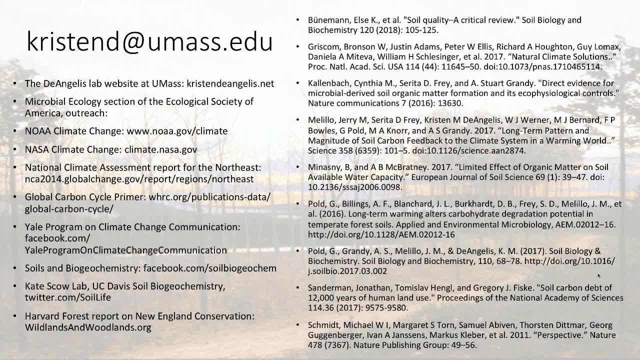 meadow into forest, so there are native plants that provide habitats for birds and animals and insects, and so meadows are super important. you know, cultivated meadows, you should have more natives- and but also this is something that's true for not just ecosystems, but for all systems- microbial systems, human, social systems that are more diverse. 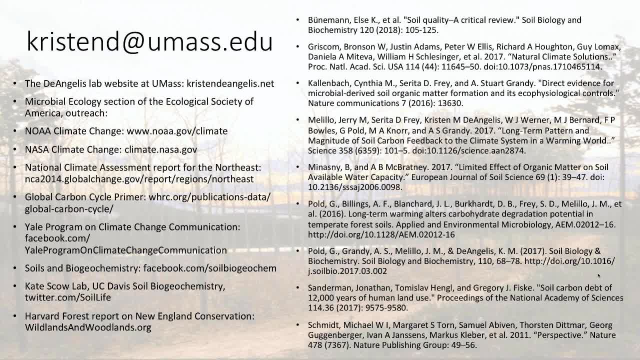 systems that are more diverse have more productivity and are more resistant to stress. That's just a fact. The data over and over show that if you have more different plants provide more different niches for more different microbes and more different animals, and those systems are more 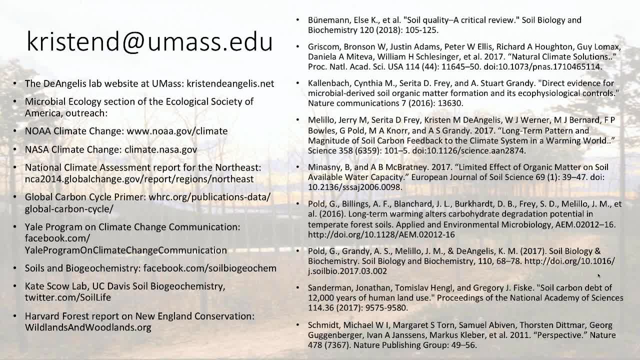 drought tolerant. they're less prone to erosion. they can withstand heavy downpours. Same is true for microbial communities. More efficient microbial communities are more carbon use efficient. They put less carbon into the air. It's really kind of amazing actually to me that you can look across different. 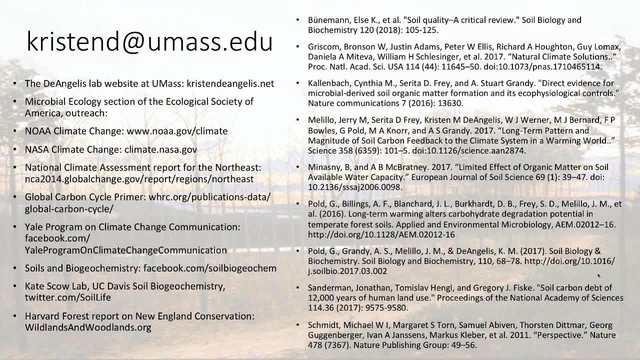 different types of living scales and still see this effect of diversity as a positive driver for stress resistant and productivity. So I don't know if that answers that really nice question, but, um, you know, I think meadows are great. I just focus on forests because that's my interest. 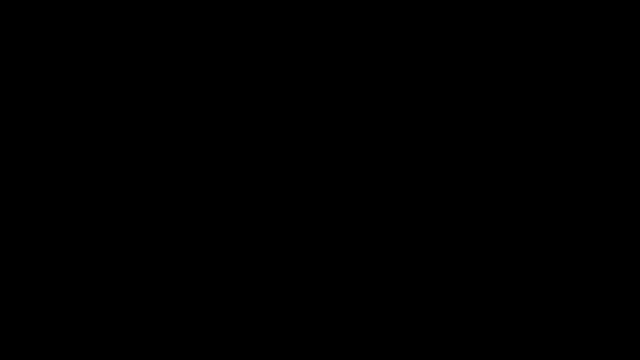 Thank you. All right, thank you. Can you suggest a couple of things that municipal park managers could do to have a positive impact? Gee, more native plants. Okay, Yeah, more native plants. I mean, I know you know there's a lot of different ways that a park can look, and 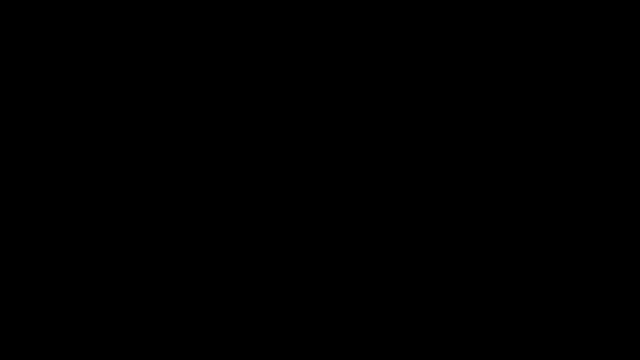 you know, big sort of lawns are pretty environmentally- I don't know how to say this without editorializing- they're not that good. They don't store as much carbon. You know you need to use fossil fuels to mow them. They don't serve as a 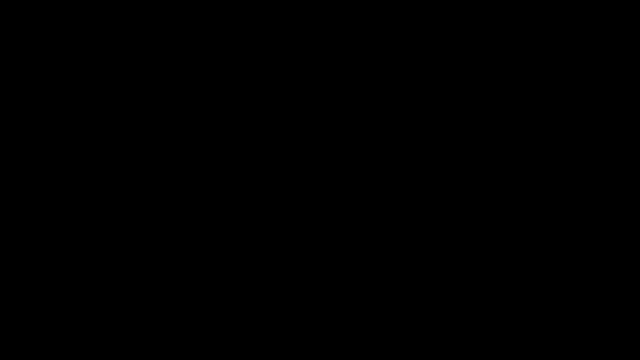 habitat for insects and animals and pollinators, as well as like wildflowers or meadows, would Um. so that would be one suggestion, I suppose. Okay, Can you explain the difference between how microorganisms may affect long-term and short-term carbon storage? 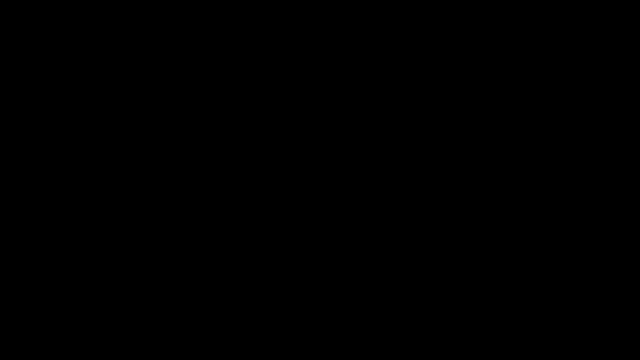 Can I explain the mechanisms of how microbes affect long term and short term? Yeah, so you know the short-term carbon storage. we can understand that pretty well and we do those takes experiments in our lab where can sort of look at like microbial exudates and how microbes interact with. 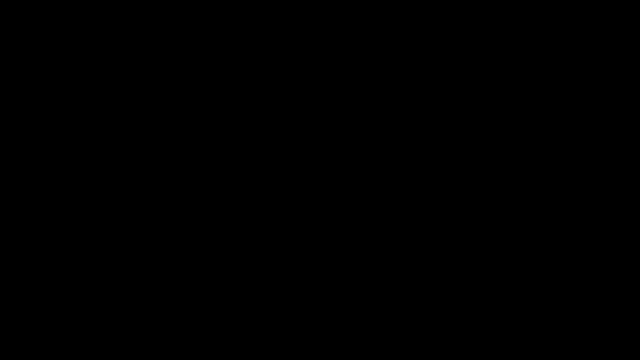 minerals, and we're not the only lab doing this kind of work. Long-term microbes, long-term microbial effect on storage, is much harder to do, because you know so, if I want to do a research study where I want to understand the effect of microbes on long-term storage, carbon storage, which, incidentally, I would like- 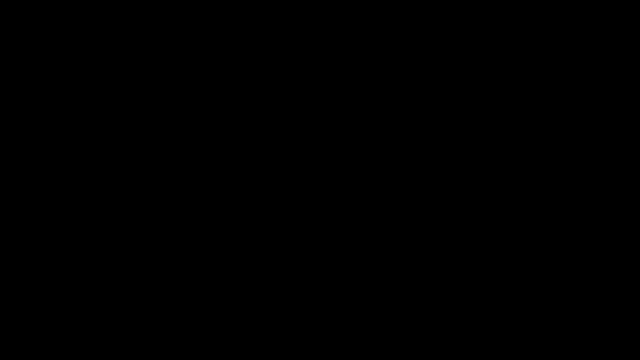 to do So. the way that I do that is that you know I write up my proposal, say: well, you know, we're going to use isotopically labeled carbon under controlled systems in the lab and we'll look at different types of soils under different types of. you know water saturation and temperatures and I might send this proposal to a funding agency like the National Science Foundation. Let's say I get lucky and get this money, Maybe they'll give me something like a $300,000 over the course of a few years, three years. 59% goes to the. 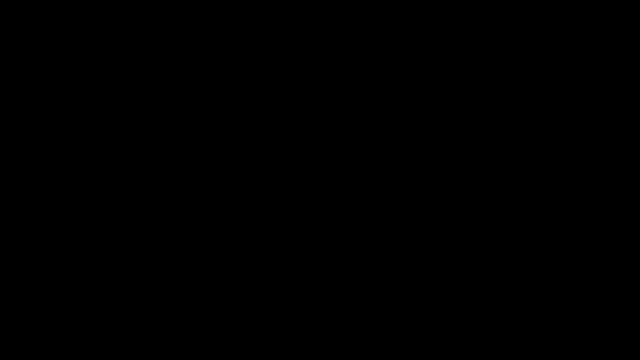 university. Almost the entire rest goes for me to hire folks in my lab like graduate students and technicians to do the work, and but then it's only for three years. So we want to know how carbon storage is affected over 10 years or 20 years, So we can extrapolate and that's something that we plan to do, and 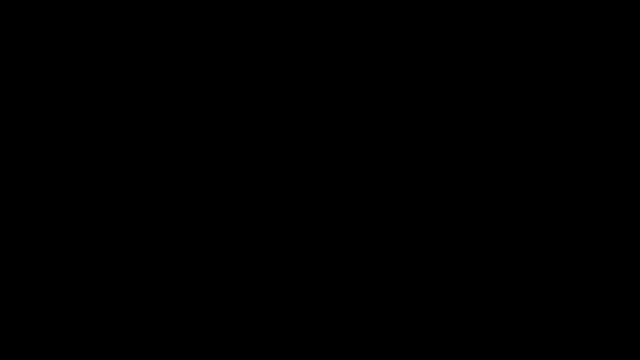 we can model, and that's actually a wonderful. utility of models is that we can use modeling to say, well, what happens over 30 years of warming, because it's not so easy to set up these long-term warming studies. So that's really the two ways right is do some modeling, or or, you know, set up a. 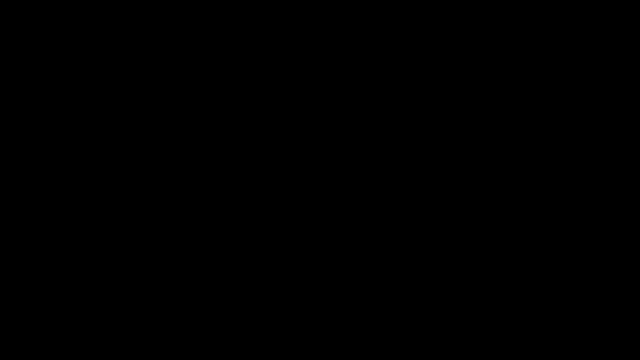 short-term experiment, that's more on the scale of the you know funding cycle, and then extrapolate using isotopically labeled carbon storage. So that's one way to do it. We labeled substrates and mixing models, So we have time for just a couple more. 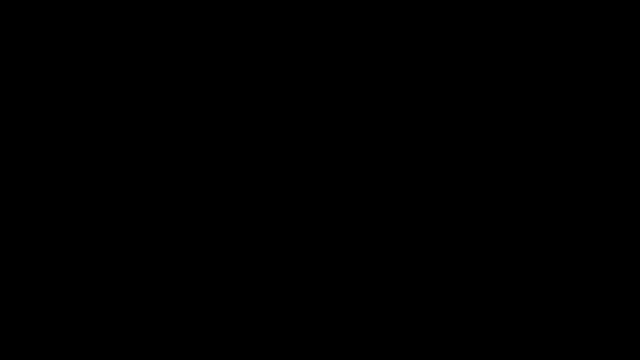 questions We are running a bit over. Is there any benefit to adding biochar to home gardens or to your client gardens in terms of carbon storage? Yeah, absolutely, and biochar was one of those 20 natural solutions, and so I would say definitely yes. Thank you so much, Dr DeAngelis, for. 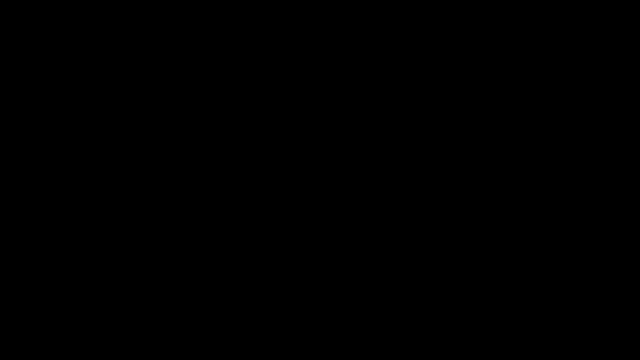 sharing this in-depth information about carbon and soil connection. This has been very, very informative, and thank you for pointing out that Google Scholar resource. That's a great way for us to learn more about peer-reviewed research for this and other topics that we're looking up, So I appreciate that. Yeah, no. problem. Thank you for your great questions.